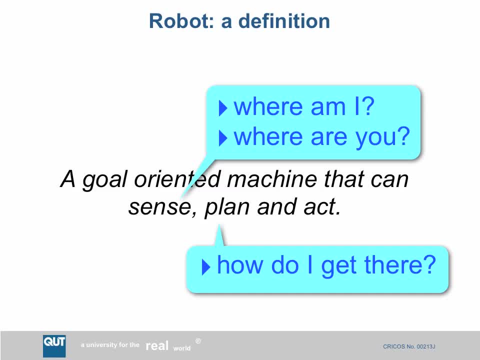 what are the important sensing problems for a robot? for a lot of tasks that a robot needs to do, the robot needs to know where it is. that's the where am I question, and it needs to know where are you. that is, where is the object that the robot needs to manipulate. 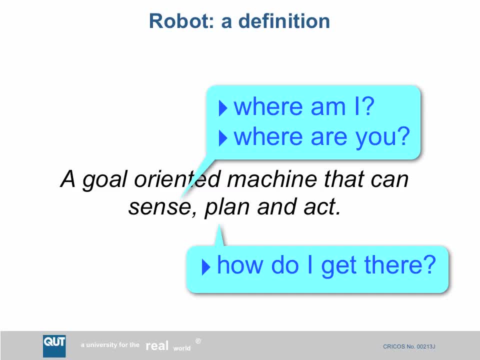 or do So. imagine that I am a robot car and I want to go to a particular place. I have to know where I am. I have to know where the place is that I'm going to, where is my destination, and from that then I. 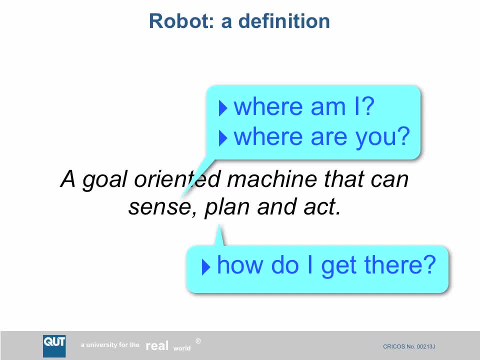 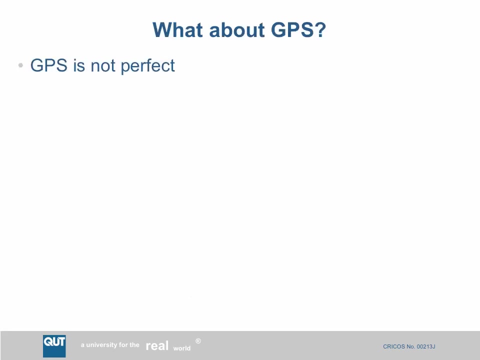 can compute a path between where I am and where I need to be. That's actually the planning problem, the how do I get there problem. Now there are many tasks where we need to perform this problem of understanding: where am I? Now, if you ask most people, how do you figure out where you are, they're going to say use GPS, but GPS is not. 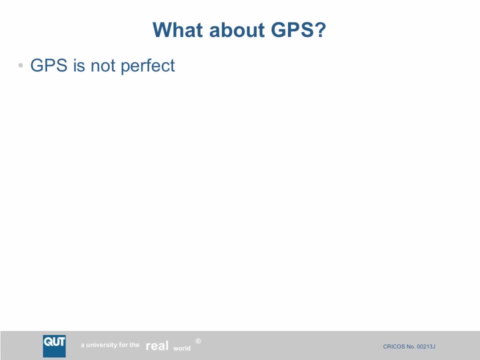 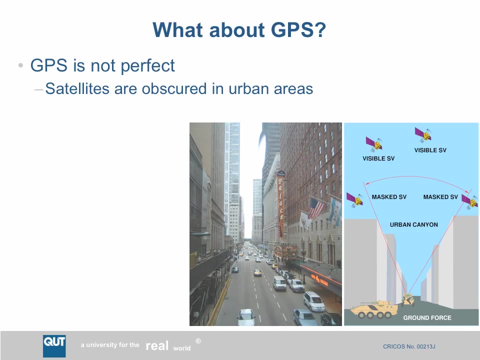 particularly well understood sensor by the general public, and it's far from perfect, and as roboticists, we're always frustrated by how imperfect GPS is. So I'll give you some examples about the infections in GPS. The first one that's important to discuss is what's called 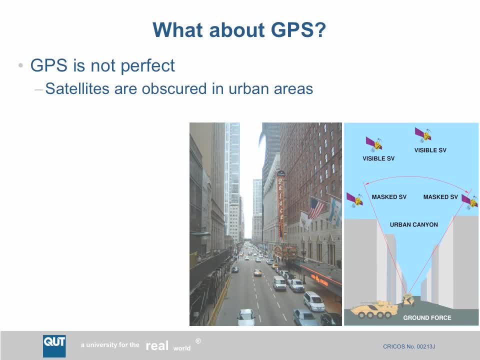 the urban canyon, and that is, if you are operating GPS in an environment with very high walls, then the satellites in the sky are mostly masked by those very tall walls. The only satellites that you're going to receive signals from are the ones that are visible above that very narrow slot. So this is a problem that happens a lot in cities where there are very high buildings, but it can also happen in mining environments. if you're in a deep mining. 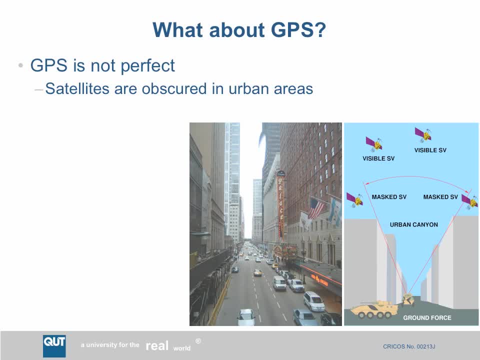 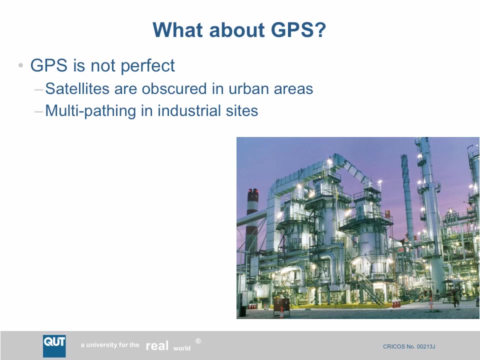 pit, Then perhaps half the sky is made invisible by the high wall of the mining pit and you can't see half the sky. half the satellites are not available to you. The chance of finding four satellites- the minimum that you need to estimate where you are- becomes much, much smaller. Another place is in industrial sites, and here the problem is that the radio waves from the satellites bounce off metal objects before they land on the 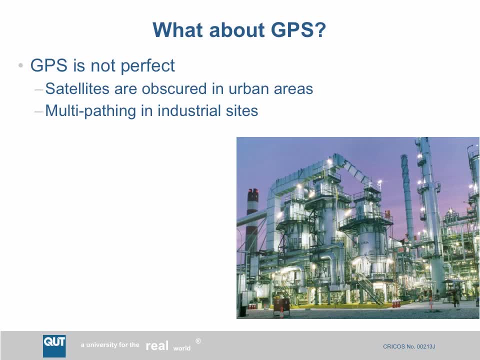 GPS receiver's antenna. Now, GPS is all about figuring out your distance from satellites in space, based on how long the radio wave took to travel from the satellite to your GPS receiver, And the underlying assumption is that the radio waves travel in a straight line. Now, if they bounce off something and then come to your GPS receiver, they've taken a slightly longer path. The GPS receiver can't know that, So when it's computing your location, it causes a horizontal display. 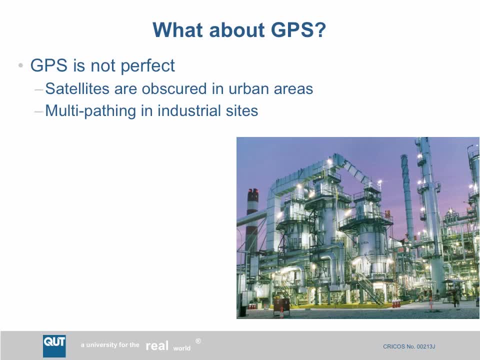 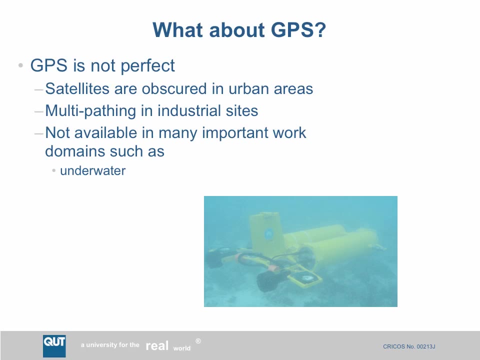 There's no way that the receiver can tell that this is the situation. So it may say that it's very confident it knows where it is, but in fact the estimate will be an error. Another situation where GPS doesn't work is underwater. The problem here is that the radio waves from the GPS satellites are incredibly weak. they've travelled a very long way and they do not penetrate water. They certainly don't penetrate salty water. they may penetrate some distance into freshwater, but they don't penetrate salty water. 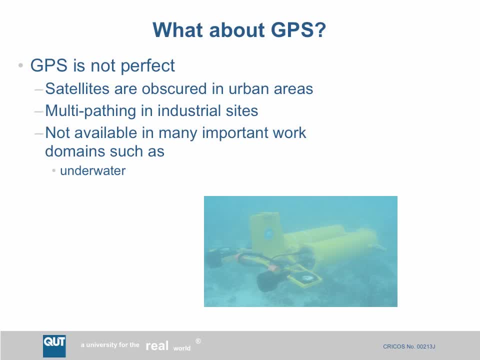 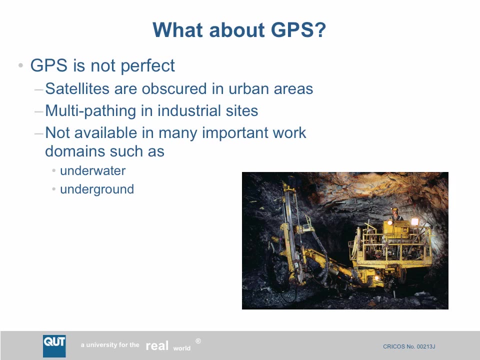 But in salty water they penetrate only a few millimetres. So if you're an underwater robot, there's no way that you can rely on GPS to tell you where you are underneath the surface of the water. Another important location for automation is underground- perhaps a mining application, And here in an underground mine, there are typically many, many machines performing many, many functions. 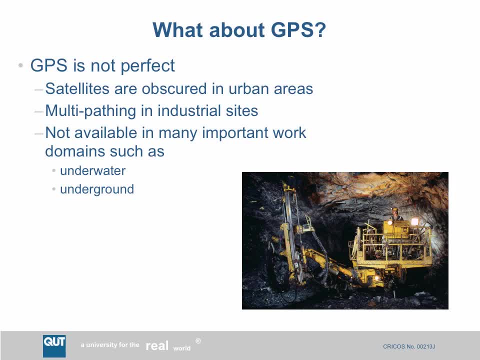 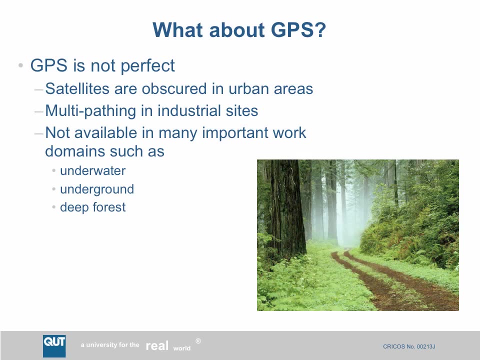 But how do they work out where they are? Again, they certainly can't use GPS, Because the GPS waves will not penetrate through the layers of rock between where the robot's working and the GPS satellites. Another area which surprises a lot of people is deep forest. 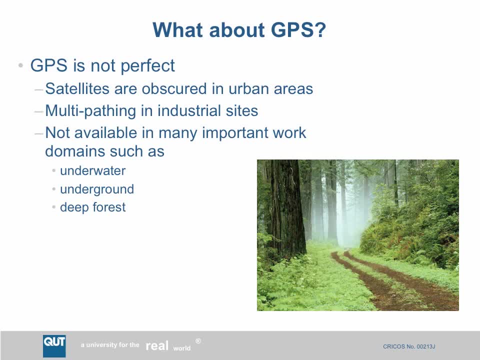 Big trees with lots of leaves- and leaves typically filled with water- absorb the radio waves the same way that the ocean does, So if you've got a big, thick canopy of green leaves above you, the chance of GPS radio waves getting through them is very, very small. 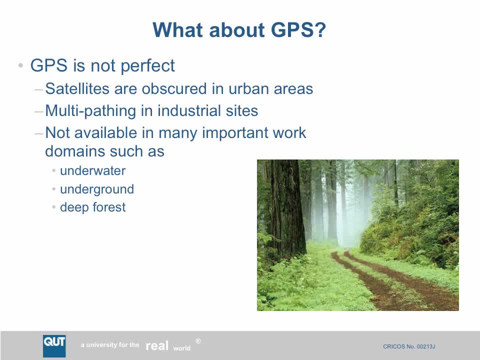 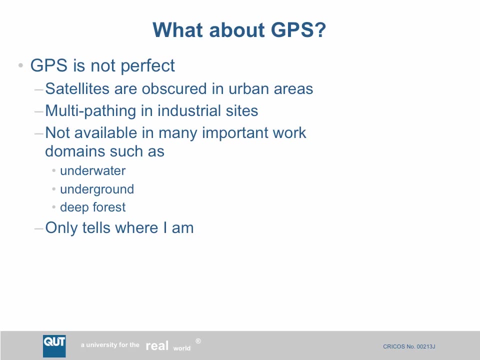 It's even worse after it's been raining or after a heavy dew. There's even more moisture on the leaves, and that reduces even further the strength of the radio waves. So there's a few reasons why GPS is not particularly useful for all robotic applications. 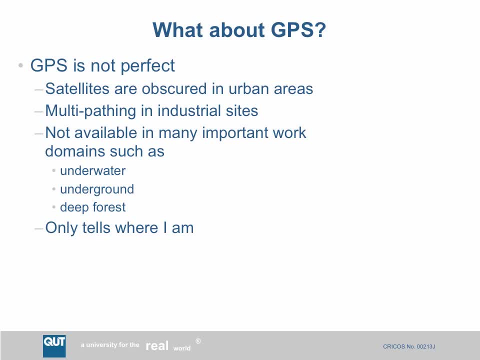 The other problem is that it only tells me where I am. If I'm a robot and I have to pick something up, it's very useful if I know where I am, But I have to know where is the location of the thing I want to pick up. 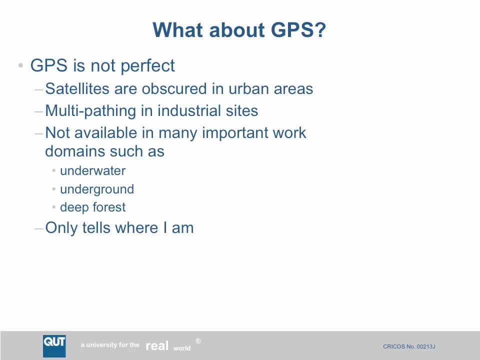 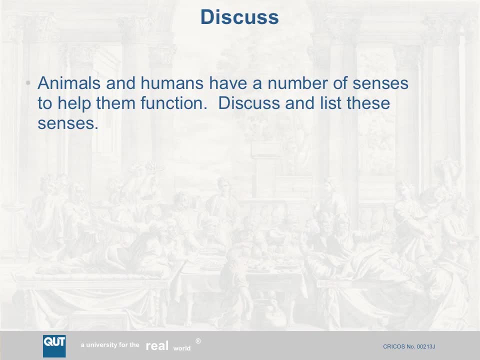 So if I'm going to follow the GPS mindset, then really what I need to do is to put a GPS receiver on every single object in the world that I might want to pick up, And ultimately that's not very practical. So, animals and humans, we have a number of senses that we use to perform all sorts of useful functions without having to rely on GPS. 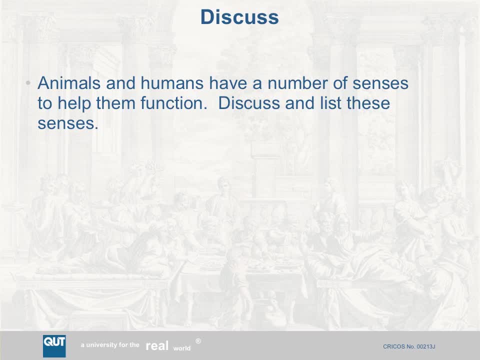 I can pick up a cup and bring it to my mouth without having to have a GPS receiver. I can pick up a cup and bring it to my mouth without having to have a GPS receiver on the cup or on me. So what I'd like you to do is to spend a few minutes having a discussion. 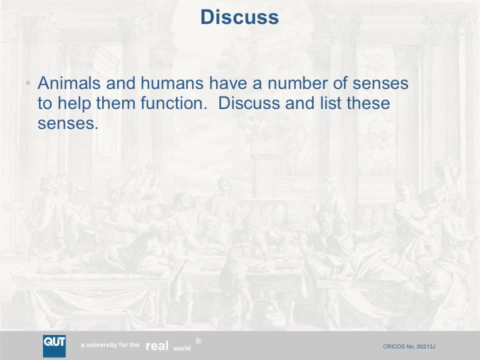 about the type of sensors that humans and animals use to perform everyday tasks, So have a discussion and list these sensors. Okay, here's my list of animal sensors. I'm going to start off with the ones that we basically learn in primary school or even. 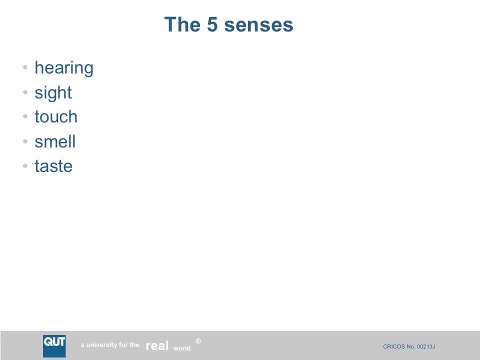 kindergarten, That's hearing, sight, touch, smell and taste. What always surprises me is that they leave out this one balance. Now, as two-legged animals, upright walking animals, the sense of balance is absolutely critical to our daily life and strangely it. 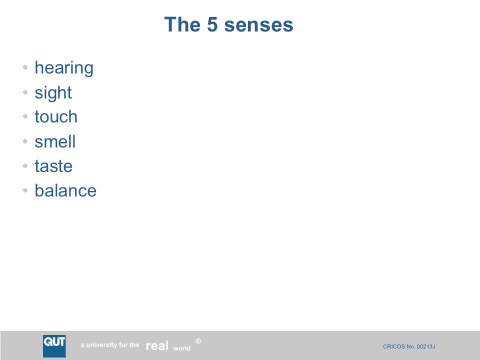 always gets ignored. Now we've got some quite complicated sensors in our body to help us with balance. These are mostly located in our body, So we're going to start off with the ones that are called the inner ear. So in your inner ear you have the semicircular. 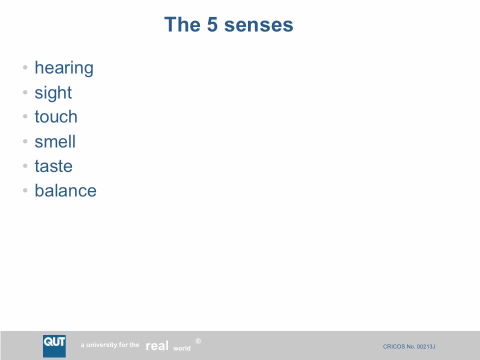 canals which function as gyroscopes that tell you about the rotational motion of your head and therefore your body, and there are also accelerometers in there, in this so-called vestibular apparatus. So in your head you have gyroscopes and accelerometers. You've 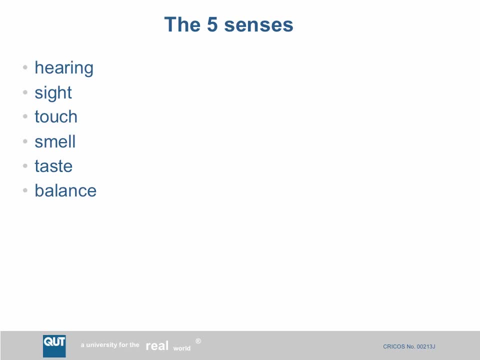 evolved these sensors and they allow you to remain upright. Now other animals have developed quite different sensors that are appropriate to the functional sense, So these are the ones that are called the inner ear. So in your inner ear you have the sorts of functions that they're trying to perform. So bats, for instance, use echolocation. 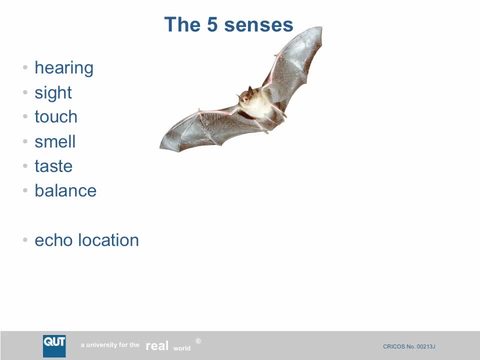 They emit pulses of acoustic energy. It balances off objects in the environment and comes back to the bat and from that it can figure out how far away an object is. But they also get some idea about the shape of the object and even about how fast it's moving and believe. 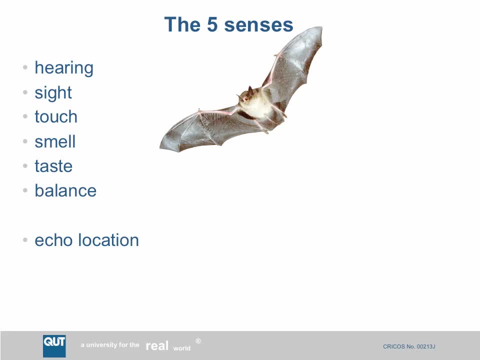 that they can even perform some sort of classification of the object. So a hunting bat can find insects and classify them and then go after the ones that it thinks are big enough or tasty enough. Other animals use echolocation as well, and I guess the best known example in the aquatic 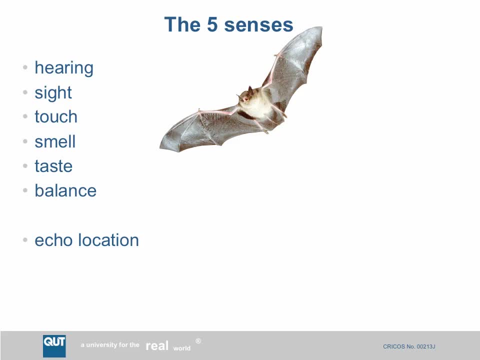 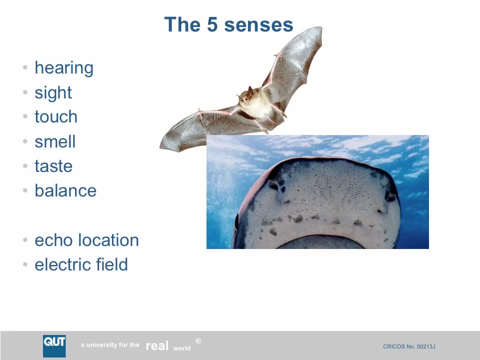 domain is a dolphin. It emits pulses of acoustic energy through the water and uses that to locate fish. Also underwater, a number of animals use electric fields, So there's little dots all over the snout of this big shark So it can pick up tiny, tiny electrical impulses from living organisms that are around it. 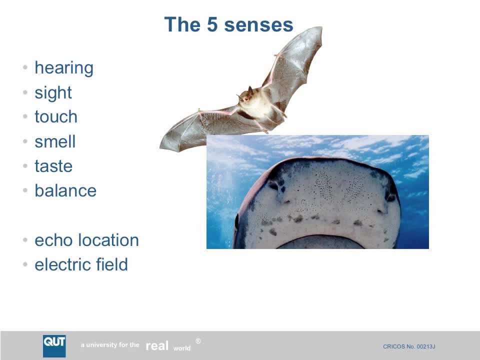 And you use that to again to classify them, work out where they are and so that it can go and eat them if they're the sorts of animals that it wants to eat. Last one that's very interesting is a number of birds have magnetism sensors in their heads. 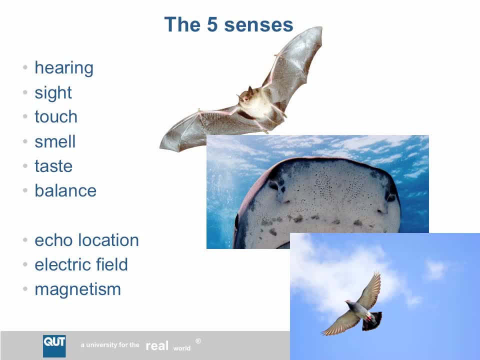 They've got a compass in their head and they use this for long-range migration, So they know where to find them, They know where to fly, which direction to fly, whether it's day or night, sunny or overcast. So these are some of the sensors that animals have evolved over many, many millions of years. 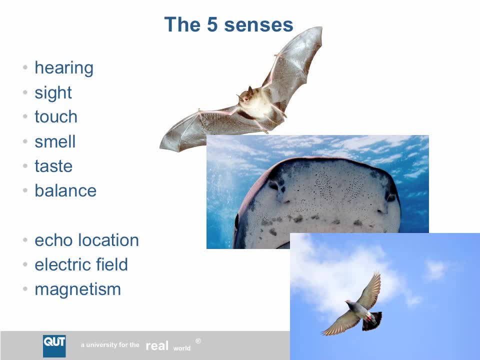 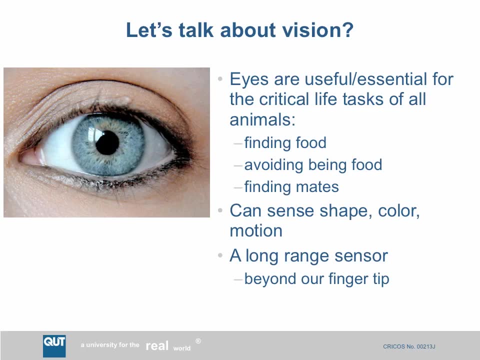 in order to perform competently the tasks they need to do in their everyday life. So I want to talk specifically about vision. Vision has always been a big interest of mine- How it works in animals, but particularly how we can try and replicate some of the functions. 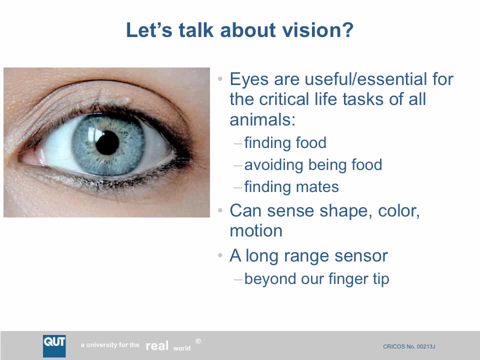 of vision for robots. So here are some things that I think are important about vision. First of all, I think eyes are useful, or perhaps even essential, for all of the critical life tasks of all animals. Vision is essential to finding food. If you're a hunter or a hunter of prey, or if you're a gatherer of fruits, you need to use vision to identify. 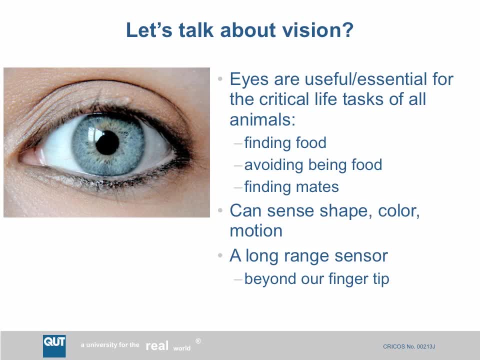 what it is that you're going to eat. It's also really helpful to avoid becoming food. So if you are an animal that might be preyed upon by another animal, you're going to use your eyes to keep an eye out for that guy and avoid it when it comes near. 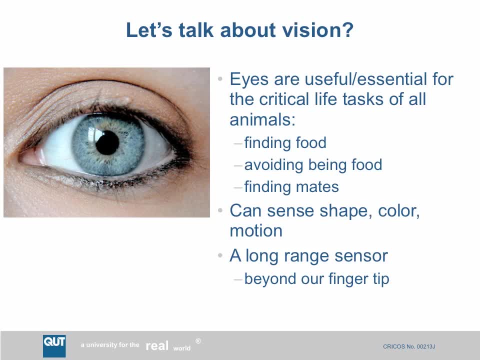 So a lot of rodents, small animals, on the surface of the ground. they're very, very good at seeing predatory birds flying above them. The other thing that vision is really important for, particularly for a lot of our animals, especially for a lot of very simple animals, is for finding mates. 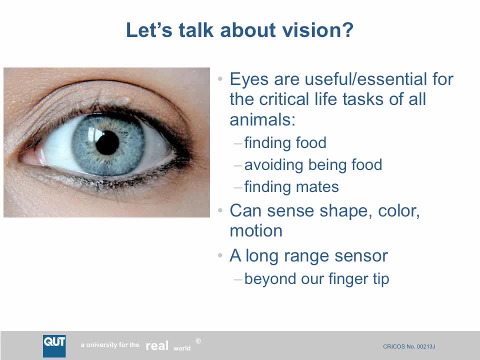 So eyes are useful for important things in life, which is essentially food and sex. Vision also is quite a rich sensor. So not only can it sense how far away something is, it can sense what shape it is, what colour it is, whether it's moving. 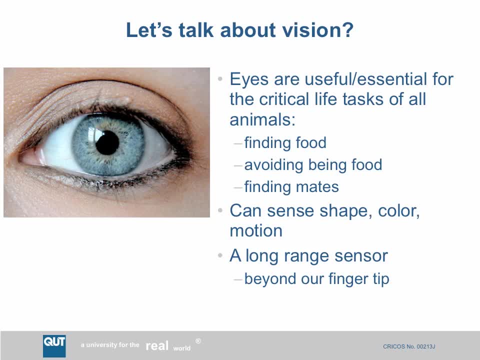 It can sense texture. So it's a very, very rich way of describing objects in history. So it's a very, very rich way of describing objects in history in our world. And the other thing that's really important about vision is that it's a long-range. 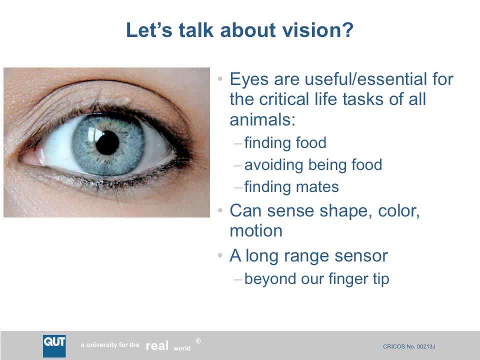 sensor. Think about all of the other sensors that we talked about earlier, particularly the sense of touch. Touch only works for something that's within our reach, So if I can touch it, then I can get a sense of feel. I can sense what it feels like, But if it's beyond my reach I can't touch. 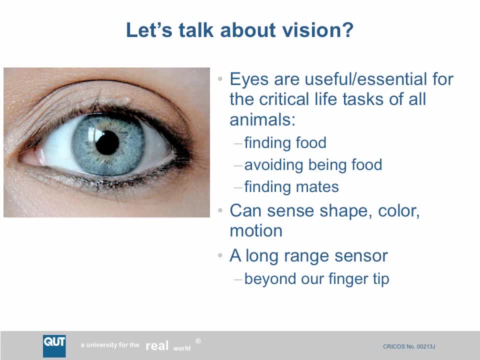 it. I can't sense what it feels like. With vision, I can see things many, many hundreds of meters away and even kilometers away. Perhaps the only other really long-range sensor that we have available to us is smell. We can smell an odor that's come from a very long way away, but most 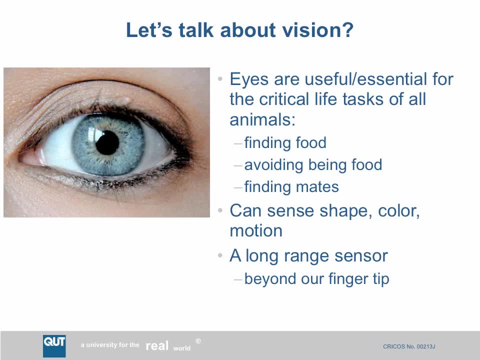 of the other sensors are very local- Touch taste, for instance. So these are the things that I think are the real advantages of vision, particularly the fact that it's a long-range sensor. So consider these two pictures. We've got the boy on the left. He's catching a ball. 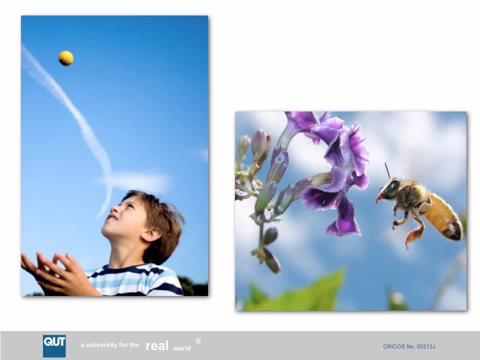 Now, going back to what I was saying earlier about how we would perhaps use GPS to solve a problem, it's clear in this picture that the boy is not using GPS, right, He's using his eyes to look at the ball. His brain is making some sort of predictions about where the ball will move. 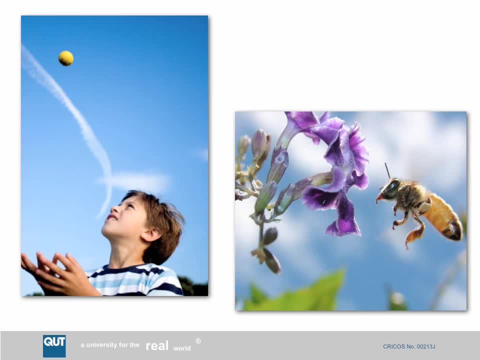 to in the future, And he's going to adjust the position of his hands so that they intersect the path. This is all stuff we do without even thinking about it. It's second nature to us, And so we can use vision to do quite complicated manipulation tasks. that is, you know, grabbing things, picking things. 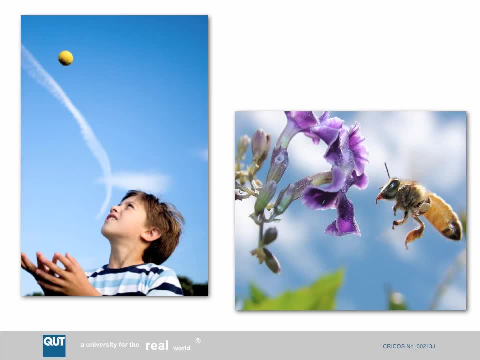 up. We do it just using vision. We don't need to know the position of the ball in some sort of coordinate frame. We don't need to know where we are in a coordinate frame. We do it in a relative sort of way, As long as I know where's the ball with respect to me and I've got some idea about. 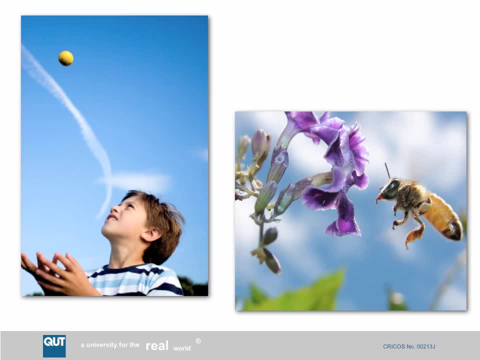 how balls move in the order of where the ball is moving. I can do it, And so we can do it in a more complex way. So if I'm looking at a human being, and I'm talking about this little animal and I'm talking about 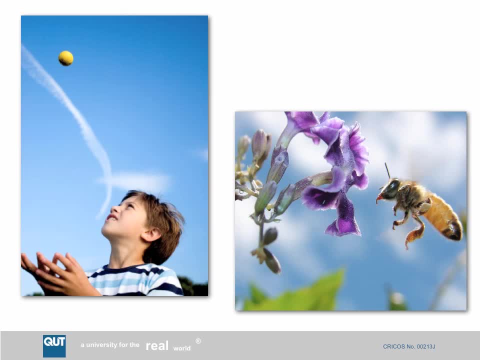 a monkey- and I'm talking about a bird that's moving in the world- then I can do some pretty complex and clever things with the ball. Now the boy there is, he has got quite a large brain and the human being, And we'll talk about 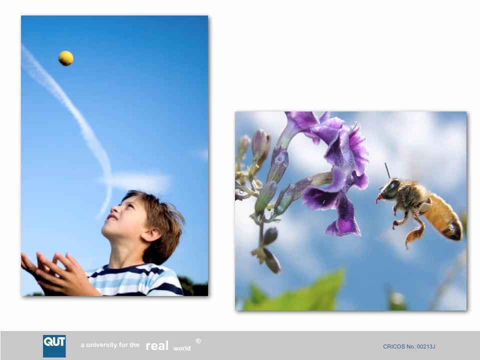 brain size in a moment. But the picture on the right shows a very, very small animal. It's a bee, And it's doing a very complicated task too. just using its eyes, What it's doing is it's going to take some nectar from this flower and it's going to land on it. It might be that the 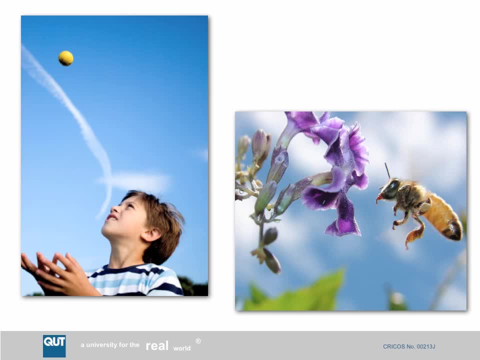 flower is moving in the breeze. The bee is going to take some nectar from this flower and it's going to land on it. The bee has got to adjust its flight so that it can land at pretty much zero velocity on the flower which is moving, drink the nectar and then move off to the next one. 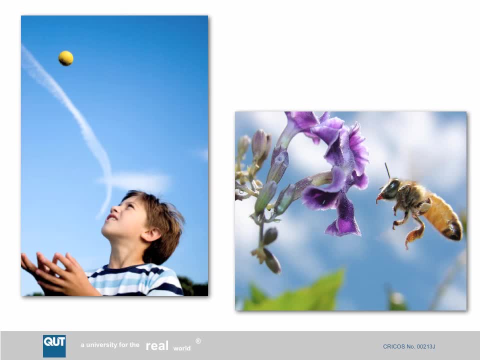 So it's using its eyes to find the right sort of things- to land on a flower, in this case, but also to control how it moves with respect to the flower. So these are two, I think, quite nice examples of how we can use vision to control the motion of animals to perform useful tasks. 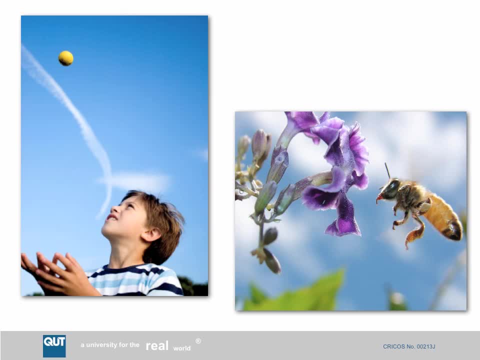 And I think our big challenge as roboticists is how do we capture some of these ideas and build them into robots so that they can perform tasks that are as functional as this. What's really astounding about the bee is that it has a very, very small brain. 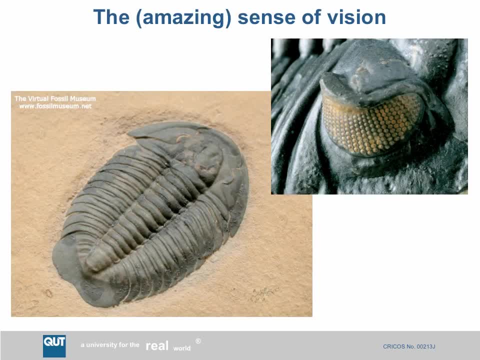 And that's an interesting fact that I'll come back to in just a moment. So vision is a really amazing sense. It evolved about 540 million years ago And life on Earth, Life, has been around for perhaps 4 billion years, But the sense of vision has only been around for about half a billion years. 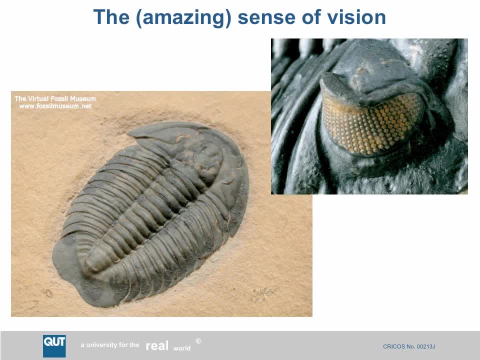 So the early organisms that lived on Earth were really very, very simple And they blundered around in the ooze And if they found something that they liked and bumped into it and they liked the taste of it, they would eat it. 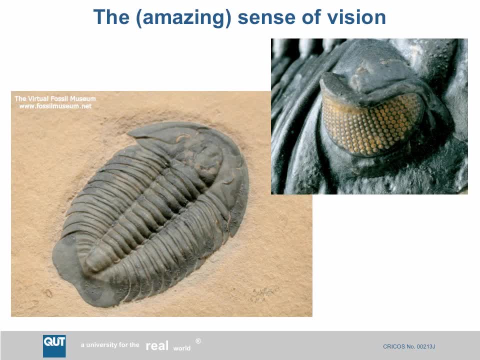 But they couldn't plan very much because they couldn't sense things that were very far away. Now that all changed when some organisms got vision, Because once some organisms got vision, then they could figure out where other things were and go and eat them. 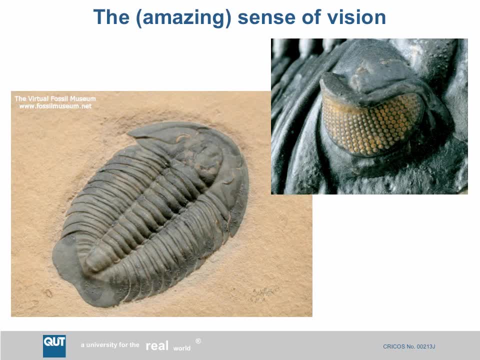 So those other organisms also evolved vision. So when they saw a guy coming to eat them, they could move away. And what happened 540 million years ago was a great arms race. So once we got vision, it made it easy for animals to prey on other animals. 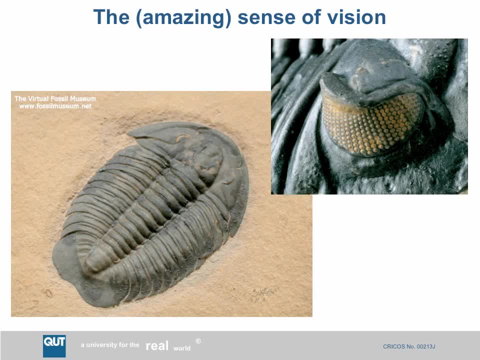 Animals wanted to defend themselves against that, So they evolved better vision. Both the prey and the predators evolved better vision, But then they also evolved armour so that they could protect themselves from predators. And then the predators evolved bigger teeth and claws. So there was this great 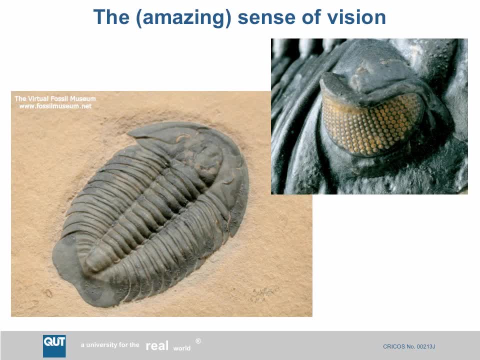 I call it an arms race, And it literally was, as animals evolved all sorts of techniques to improve their position with respect to other species, And it was this sense of vision that I believe, really ignited this whole process. So for many billions of years, life on Earth was pretty dull. 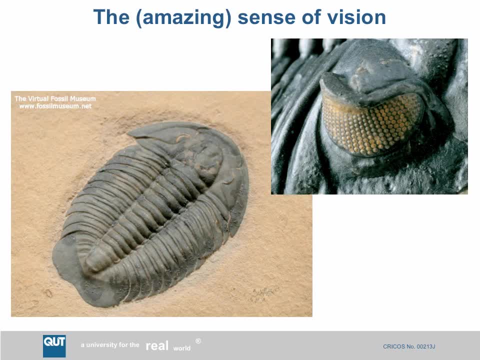 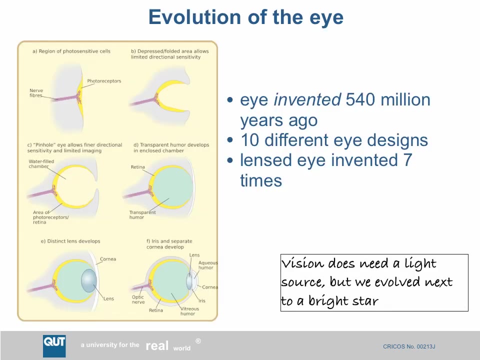 Vision came along and suddenly it all changed. We had what was called the Cambrian explosion. A huge number of things happened, A huge number of species evolved, And that kicked off evolutionary processes that led eventually to us being here in a classroom at QUT here today. 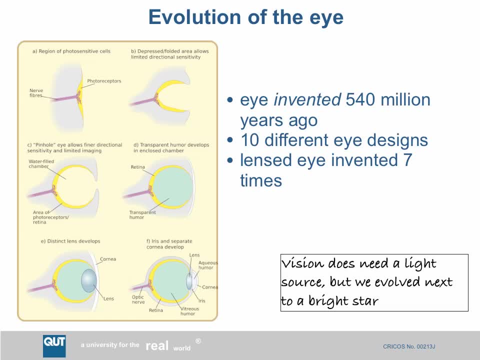 What's interesting, too, is there's been a lot of speculation about how the eye evolved, And the speculation is that we developed some cells that were a bit sensitive to light on the surface of the body And that eventually, this patch of what we call photoreceptors- light receptors- 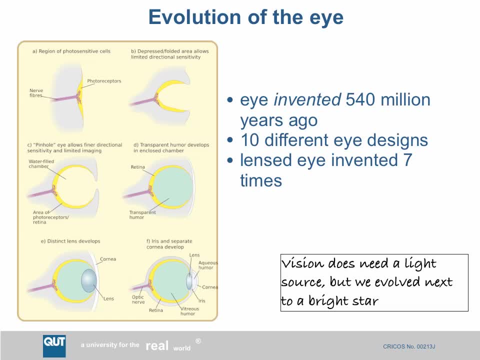 turned from being a flat patch to a cup, And the advantage of it being a cup is then photoreceptors had some better idea about which direction the light came from- Not that there was light or not light, but which direction it came from. 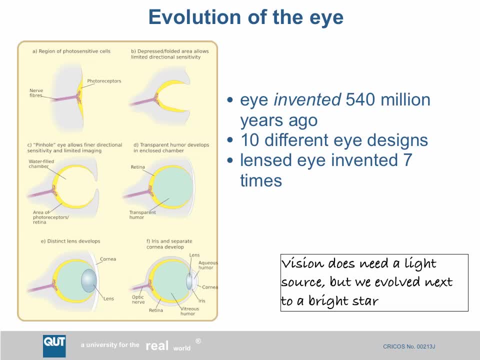 And eventually this cup folded right over and became almost a closed sphere. It then filled up with transparent liquid, A lens evolved, And then some other apparatus to control the amount of light going in and out The iris, And we have the modern eye. 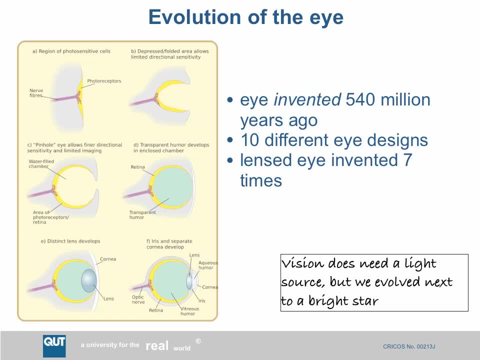 What's really interesting is that the eye has been invented, it's believed seven different times independently in evolution across species, And that there are ten different designs of eyes around in the world. So it's not just the lens eye that we and most mammals have. 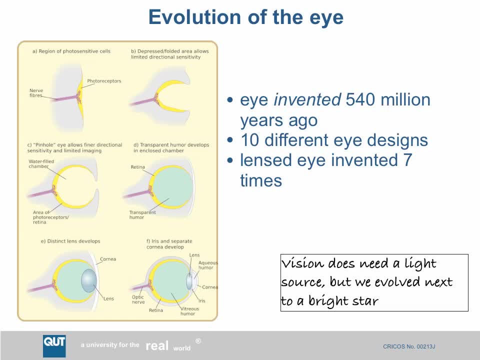 There are all sorts of other eyes that exist in nature, So I think the fact that the eye has evolved- The eye has evolved so many different times with so many different designs- really indicates that it's a very powerful sensor. Animals get a lot of benefit from having this sense of vision. 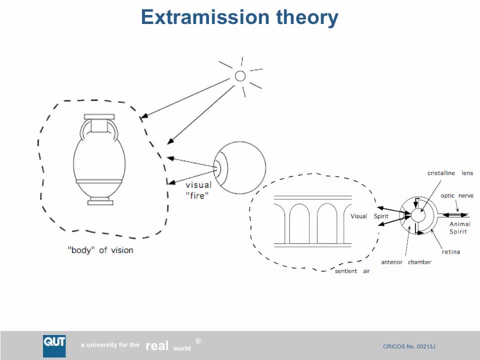 And that's why it has evolved Now. not so long ago, in the time of the ancient Greeks, they didn't have a really good handle on how vision worked, And what they believed was that the eye emitted a substance. They called it visual fire. 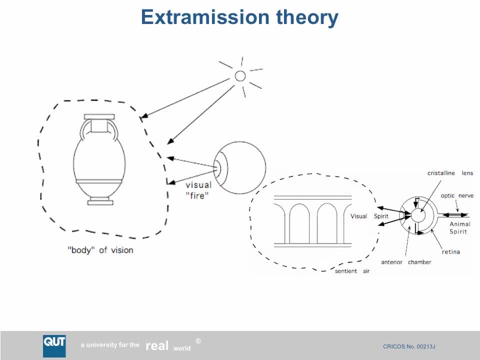 And what it did is it left your eye and it went out and it interacted with objects in the world And what you saw, they believed, was analogous to touch Where this visual fire went out and intersected an object. you felt that. 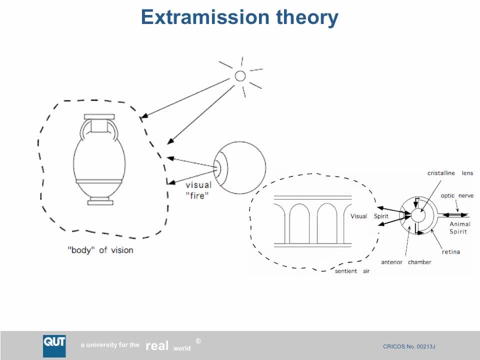 And that feeling is what we see as vision And it's called the extramission theory, And it took quite a long time to turn this theory over. And the theory that we have today is that light from some light source, like the sun, lands on an object, it reflects off and comes into the eye. 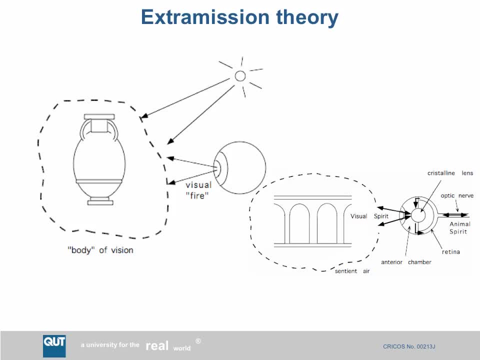 where it's converted through a chemical process into electrical impulses which go into our brain, into our visual cortex and cause a visual perception. So the model now is that the light is coming into the eye. but this extramission model was that some mythical substance left the eye. 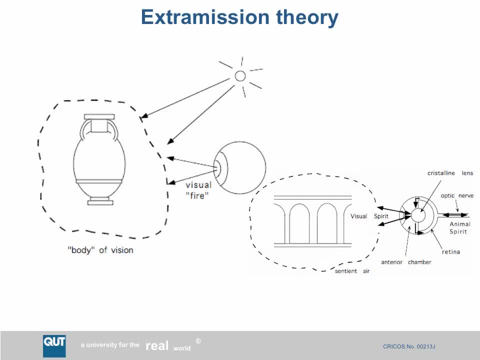 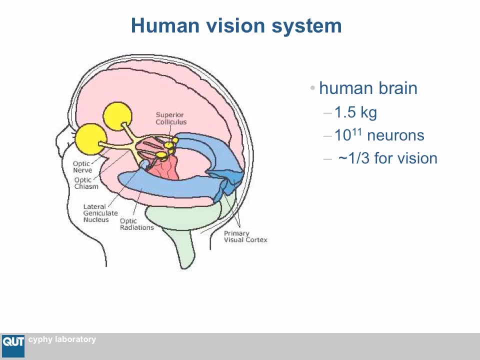 went out, interacted with the world And we felt that. So the human vision system is a substantially large part of the human brain. We've got large brains. Our brain weighs on average 1.5 kilos. Nearly one third of that is used for vision in the visual cortex. 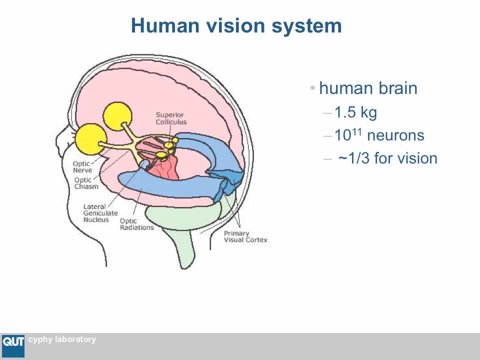 So that's half a kilogram of meat in your head- is involved in visual perception. We have a lot of neurons in our brains. We have 10 to the 11 neurons. That's a very, very big number. It's interesting too that the visual cortex 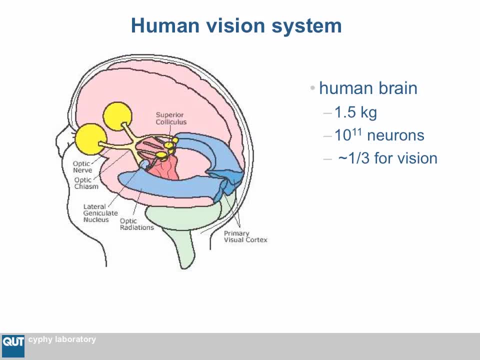 isn't where you think it would be: at the front of the head, near your eyes. It's actually at the back of your head And there are these long optic nerves between the eyes at the front of the head and the visual cortex at the back of the head. 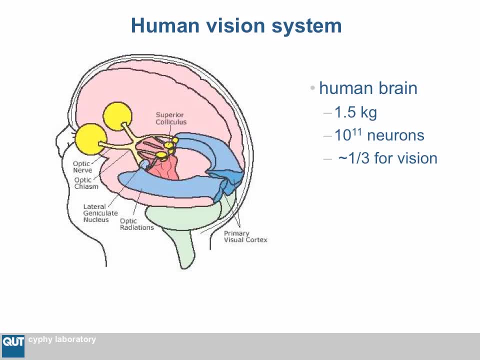 And a side effect of this is if you get banged on the back of the head, you see lights, you see stars, and that's because you're getting banged on your visual cortex And that's getting misinterpreted as visual perception. So, human visual system 10 to the 11 neurons. 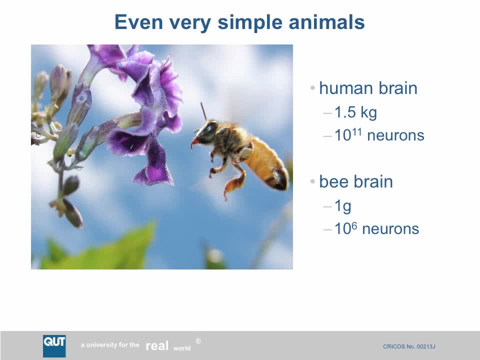 That's a very big number. Now consider the bee. We talked earlier about how the bee can do quite a complex task. It can find the right sort of flower to land on. It can land on the flower, It can go back, take it back to the hive. 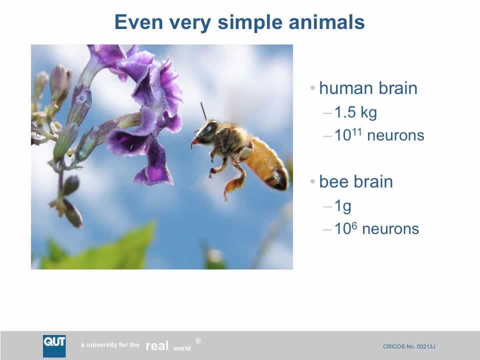 It can do a dance to tell other bees where the flower is. It's pretty clever stuff. The bee's got a tiny brain. Bee brain weighs just one gram. It's got only a million neurons. So very small animal, very simple brain. 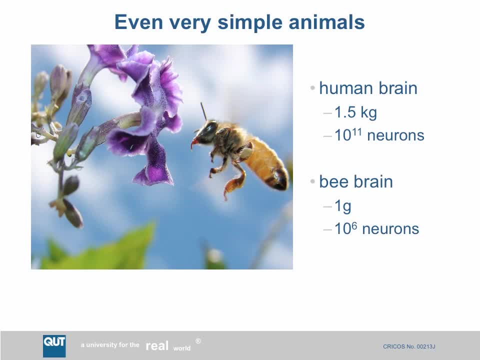 but it can do quite complicated things. It can do complicated tasks just using vision. And this is where it gets exciting for roboticists, because 10 to the 6 neurons is not very much. A neuron doesn't do very much computing. We've got computers now that have got more computing power than a bee's brain. 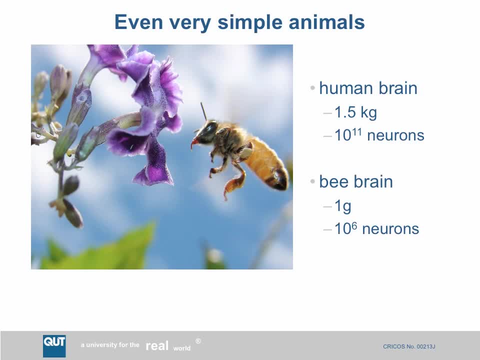 What we don't have, though, at the moment, is really the right way to use that computing power to do a task that's quite as clever as the bee. There are lots of people right now looking at this problem. Roboticists are looking at this problem. 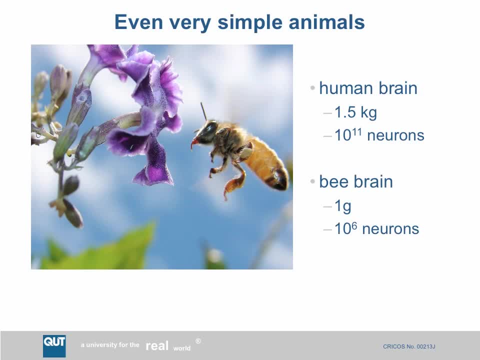 and a lot of insect scientists are looking at this problem as well, And sometimes there are groups of insect scientists and roboticists working together to try and see how we can borrow, steal the techniques that simple animals like bees use, build that capability into robots. 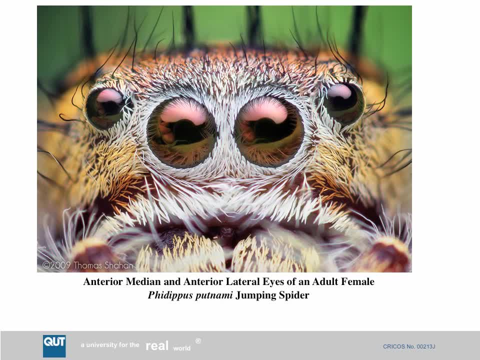 So here's a picture of the eyes of a spider, And so you can't assume that all animals have two eyes. All mammals have two eyes and insects like bees have got two eyes, But it doesn't have to be two. So here's a picture of a spider. 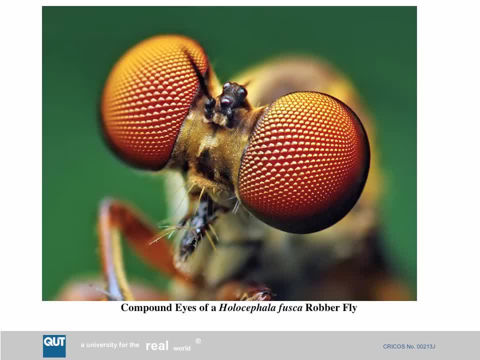 And this particular spider's got four eyes, which has been interesting, And here's a picture of a robber fly And you can see that it's got these very bulbous compound lens eyes And I'll talk in a few moments about compound lenses. 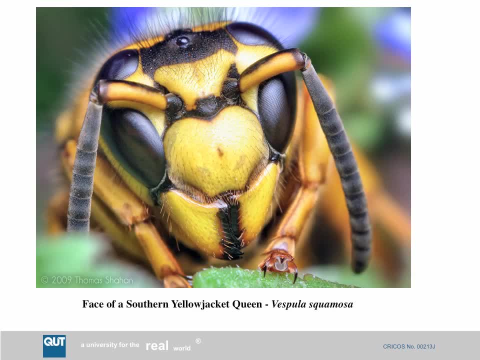 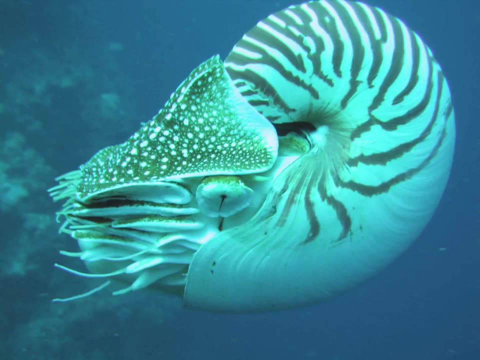 Here's another one, a waspy thing, And you can see that it's got flatter compound lens eyes, almost four eyes, But I think it's actually one continuum of compound eye on each side of its head. Here's another very primitive animal. 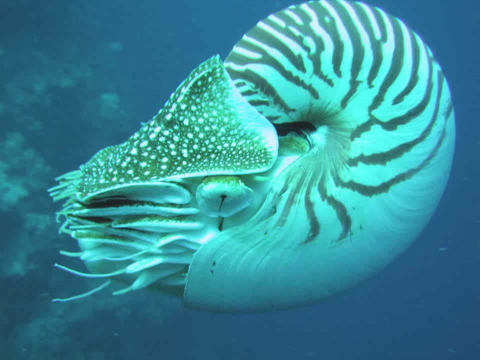 This is a nautilus. It's an aquatic animal like a big snail And it has an eye that is really like a pinhole camera. It doesn't have a lens as such. It's got a tiny little hole that the light enters. 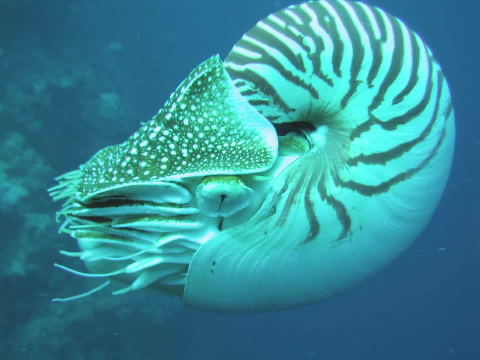 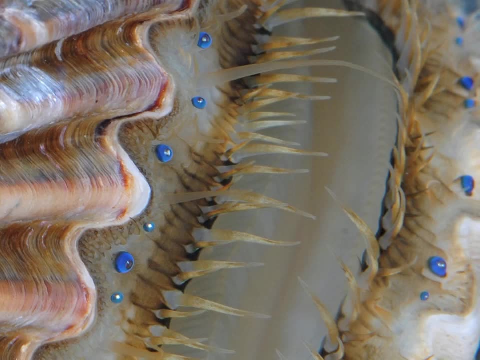 And we'll talk about pinhole cameras in a lecture later in this panel. And here's a scallop. This is a really, really excellent example of an animal with more than two eyes, So each of those blue things that you can see there. 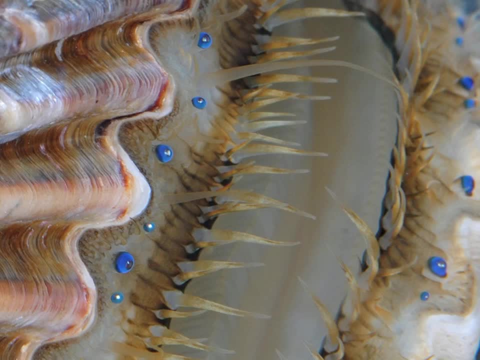 they look a bit like blueberries, are actually its eyes And it's got a whole row of eyes on either side of the shell or its mouth, And each of those eyes is quite unusual in its own right. It's actually each of those eyes is a bit like a reflecting telescope. 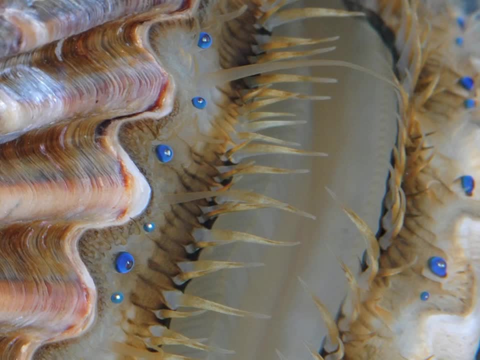 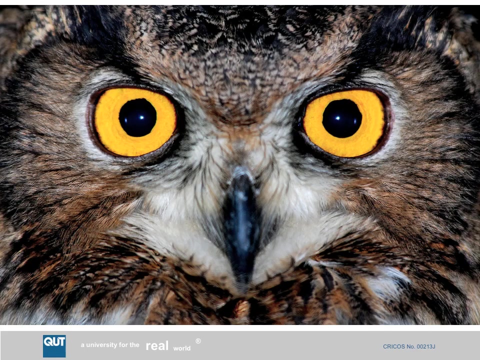 It's a hollow sphere that's shiny on the inside And the light enters the hole in the front, reflects around and lands on a photoreceptor. So simple eyes, but a lot of them, And here's a cuttlefish. 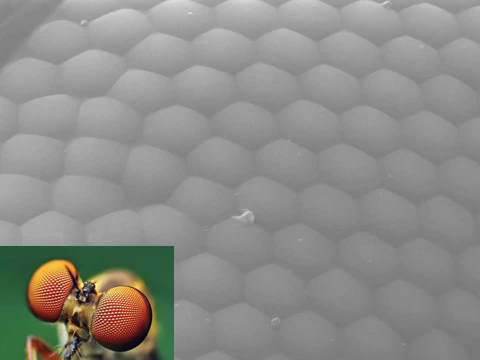 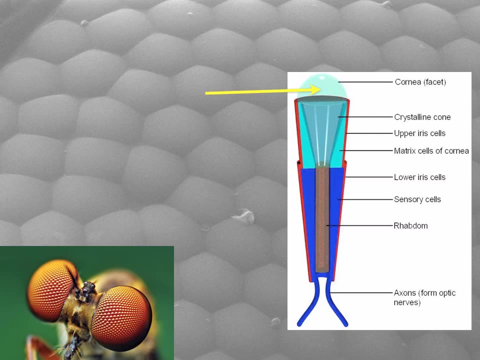 And it's a lovely picture of a bird eye. So here's a compound eye up close. Each of the little cells or little facets in the compound eye is actually an individual light sensor, So each one of those cells senses light. So on the top is a little lens. 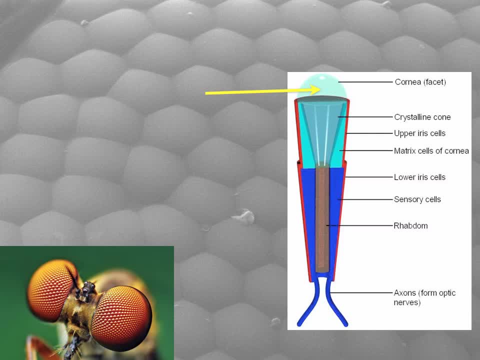 And inside then are some chemicals that convert the incoming light to electrical impulses, which then leave through the nerves out of the bottom there. So think of it as a whole lot of individual photodiodes or phototransistors or something arrayed around a sphere. 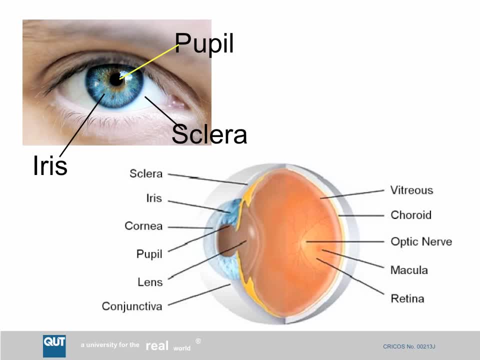 The human eye is quite a complex device And the principal components are shown here. The pupil is the hole that the light shines through and lands on the back of the eye on a surface which is known as the retina. Around the pupil is the iris. 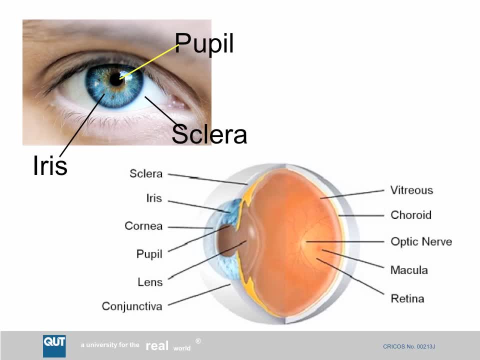 That's the distinctive colour in a person's eye And, as you well know, the iris opens and contracts and controls the amount of light entering in through the pupil. So the pupil can be small. the pupil can be very large. The area around the iris, the white part, is called the schlera. 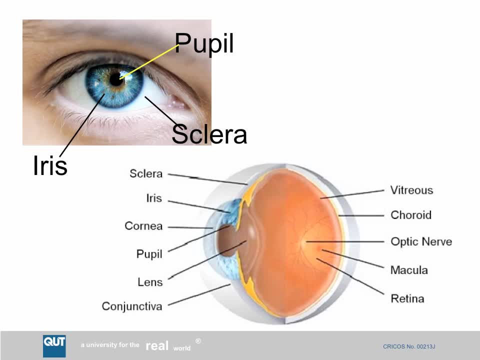 And that's part of a protective membrane that goes around the eye and actually around the optical nerve. In fact, it's part of the same membrane that protects your whole brain. In some ways, your eye is actually an extension of your brain. It's a part of the brain. 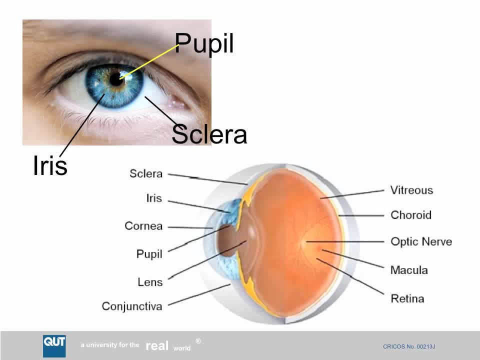 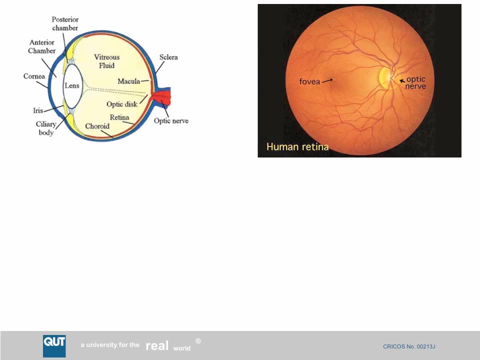 It's inside the same brain protective membrane. It's just located at the front of your head And it protrudes out of your body, But you think of it as part of your brain. Now, if we look at the side view of the human eye, 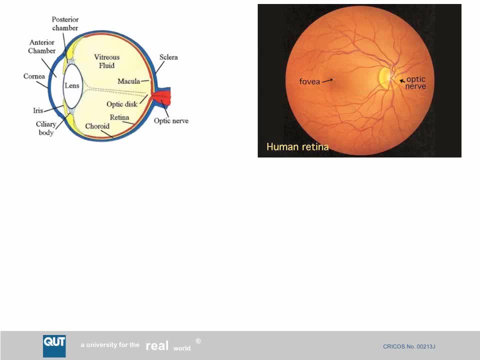 we see the lens there which focuses the light, And we'll talk about how images are formed and focusing in a future lecture. The light enters from the left, is focused by the lens and lands on the back surface, the so-called retina. 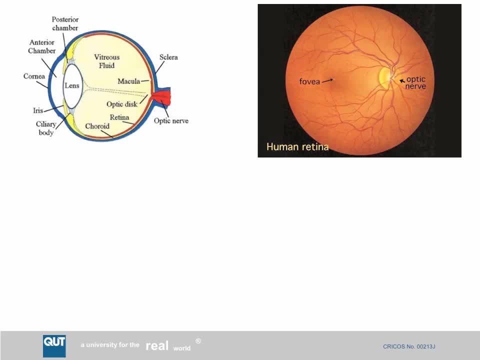 The picture on the right is a photograph of the retina And there are two distinctive parts of the retina. The first distinctive part is called the fovea. That's where there is a huge concentration of light-sensitive cells. There are light-sensitive cells all over the retina. 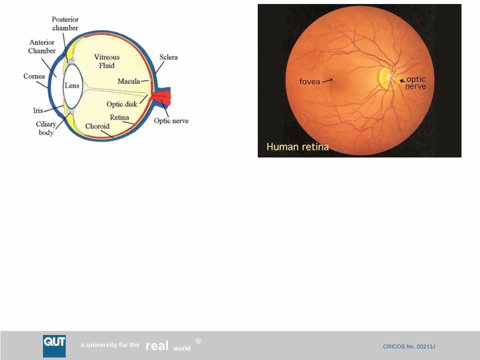 but there are a huge number concentrated in the fovea. It's a high-resolution part of your visual field, in the middle of your eye. The other very distinctive part is what's called the optic nerve, And you have to say that the human eye. 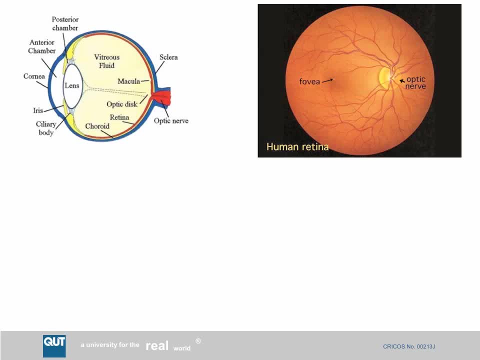 is not particularly well built, So where the optic nerve is, there are no light-sensitive cells, And so this means that actually there's a part of the retina where you can't see anything. You can see stuff very, very well in the fovea. 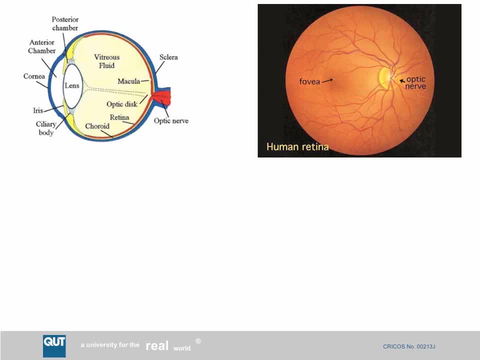 You can see stuff fairly well over most of the retina, But where the optic nerve joins the eye, you can't see anything at all. It's related to a phenomena called your blind spot, And I'll talk about blind spot in just a moment. 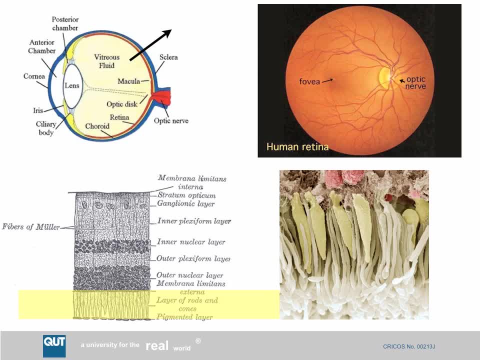 The other reason that the human eye I don't think is designed very well is that the light-sensitive cells are on the reverse side of the retina. So the light comes into the lens, shines onto the surface of the retina, But the light-sensitive cells 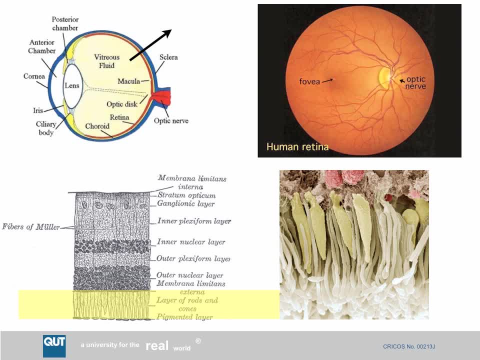 you've probably heard of these rod cells and cone cells and they're shown down in the bottom right of the screen. they're actually a few layers down inside the retina, So the light that lands on the retina has to penetrate through various layers. 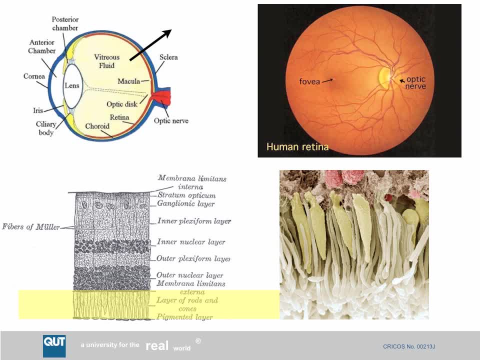 of fibres and nerves and blood vessels before it eventually lands on the rods and cones which get excited and respond to the light. So again, not particularly good design. Looking at the picture in the bottom right again we see the rod and the cone cells. 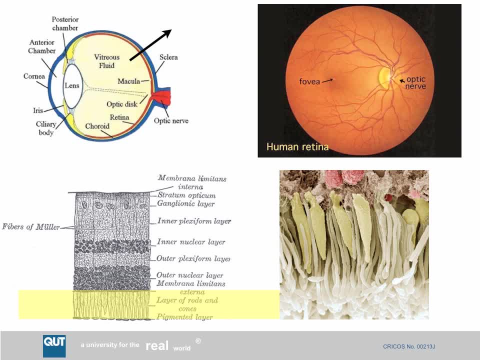 And you can see that. the rod cells are the very small, quite light-coloured cells that are very narrow. They look like worms. The bulkier cells, they're the cone cells, So the names that have been given to them are somewhat sensible. 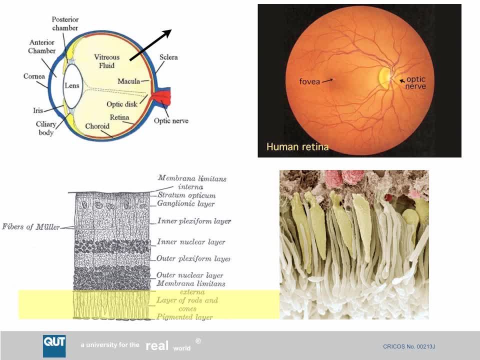 Some are a bit rod-like and some are perhaps cone-like. The cone cells are certainly much bigger Now. the cone cells are the ones that respond to different colours. The rod cells don't see colours at all, They just see light. They're also much more sensitive than the cone cells are. 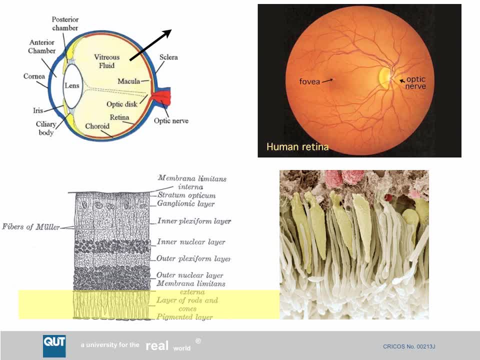 So we use our rod cells in low light and at night and we use our cone cells for colour vision during the daytime, And we're going to have a whole lecture where I'm going to be talking about colour and how that works. So I mentioned before that the fovea. 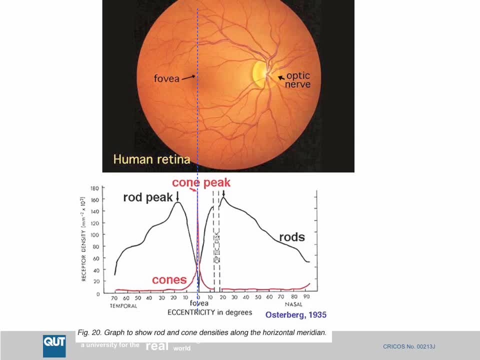 has got a really high concentration of light-sensitive cells. So this graph is a little bit busy. But what we have across the bottom is a graph that shows the density of photoreceptors And what we can see. I've drawn a dashed line there. 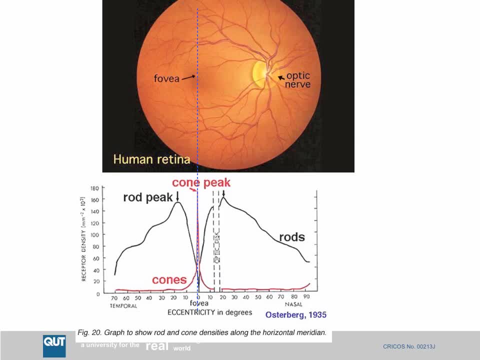 down through the fovea And you can see that there's a very sharp and very, very narrow peak In the density of cone cells. So in the fovea of our eye we have a huge number of cone cells per unit area. 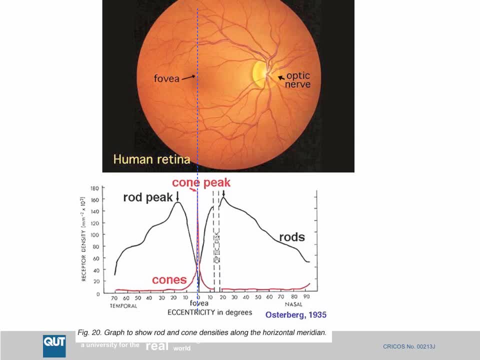 But for the rest of the eye we have very few cone cells. The rod cells are almost the opposite. We have a smaller number of rod cells in our fovea, but we have more rod cells as we move away from the fovea. 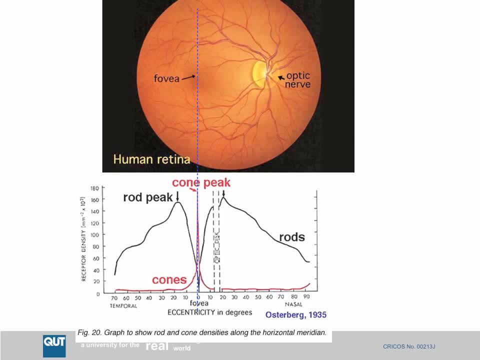 Now, another thing is that the rod cells are quite sensitive to motion, So we have a lot of motion-sensitive rod cells around, away from the fovea, in our peripheral vision area, And I think this is very useful from a protection point of view. 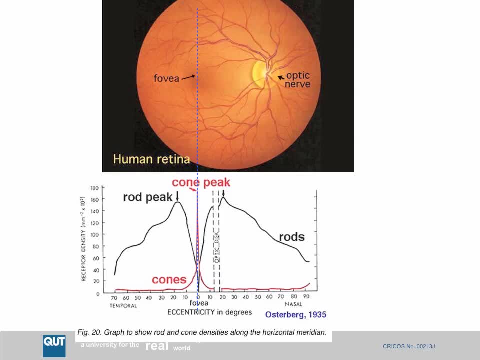 that we can see things out of the corner. we can see motion out of the corner of our eye that alerts us to something that might be a threat to us. So this is the way our eye has evolved: It's high resolution- fovea. 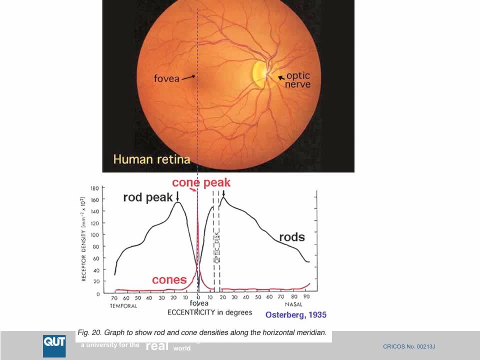 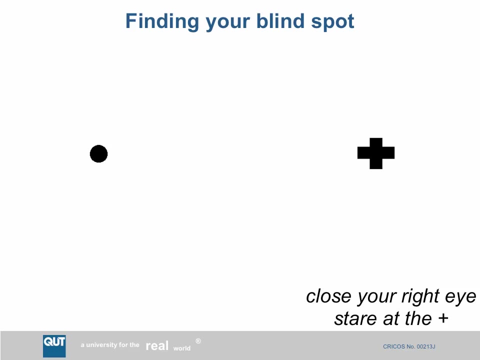 and particularly sensitive to colours and a lower level of resolution over the larger retina. Now I mentioned before about the blind spot, And again as an example of a piece of bad design. So if you go hunting on the internet, you Google how to find your blind spot. 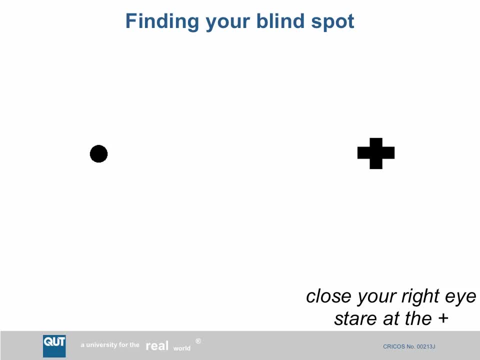 you'll find a number of YouTube videos and charts and things like that, But this is an interesting one, And if you put this slide up on your own computer and look at it, you can perhaps find your blind spot. So what you do is you close your right eye. 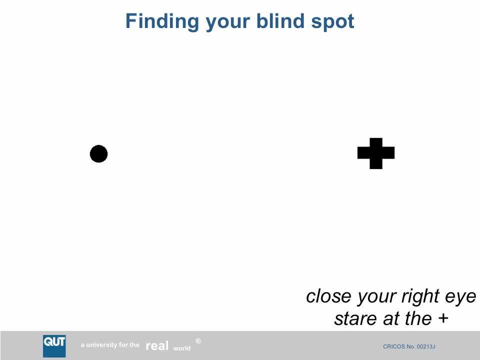 and you stare at the cross and you move your eye, your whole head, closer to the screen. So you're staring at the cross but you're aware of everything else that's in the field of view And as you move your head towards the screen. 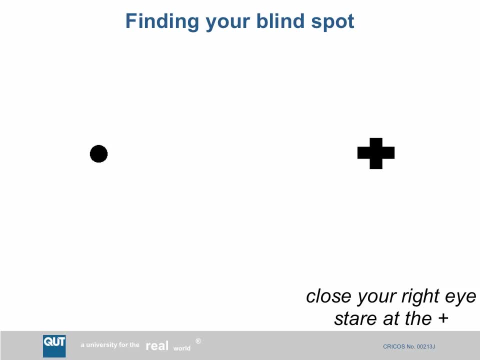 at some point you can't see the circle anymore. It just disappears. You move your head back a bit and the circle comes back into view, And what's happening is the geometry is such that at that particular point, that circle lands is being projected onto the part of your retina. 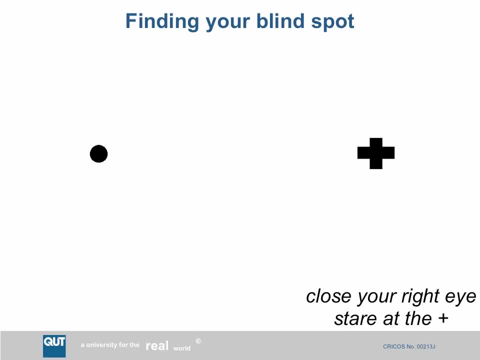 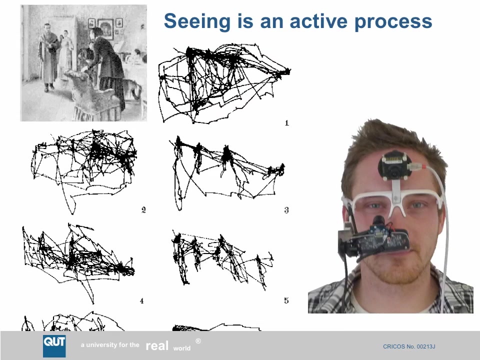 where the optic nerve enters the blind spot And you just can't see it. It's really quite amazing. So if you get a chance, have a go at trying to find your blind spot- It's a good party trick- And show it to people who are not aware of this thing. 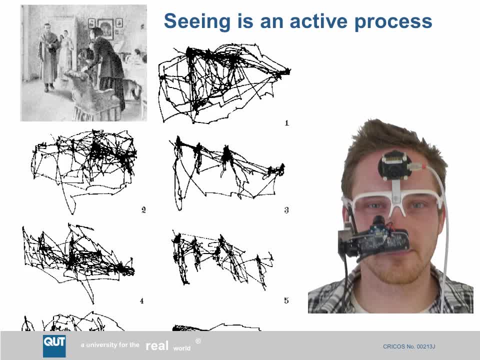 Now, the fact that you've got a blind spot- but you've probably gone through your whole life without knowing you have a blind spot- is because your eye does quite amazing things. Your eye doesn't just gaze at the world in a passive sort of way. 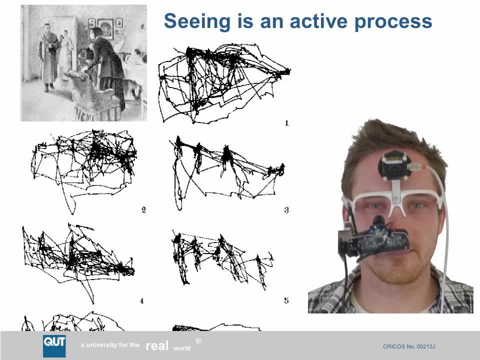 Your eye is looking at the world in a very active way, So your eye is continually darting around the world looking at things that are of interest, And you do this completely unconsciously, And this is the reason why we don't notice that we've got a blind spot. 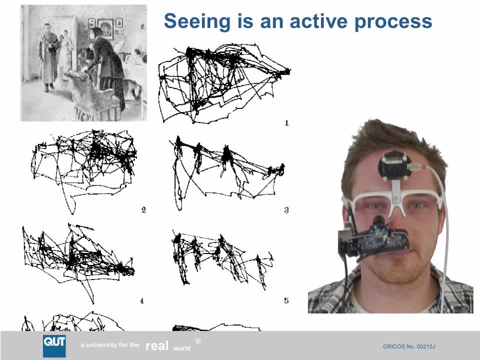 It's also why we don't notice that we've got a high resolution part of our eye and a low resolution part of our eye, Because our brain is pointing that high resolution part of the eye all around the world And so what we think we see. 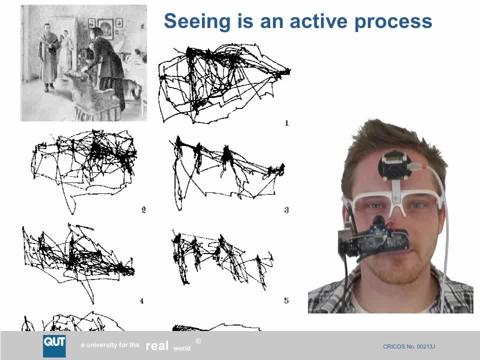 is actually a composite image built up from signals from the eye recorded as it's pointing in all sorts of different directions. So in this slide what we see is a picture up in the top of some people in a room, And it's a pretty low resolution picture. 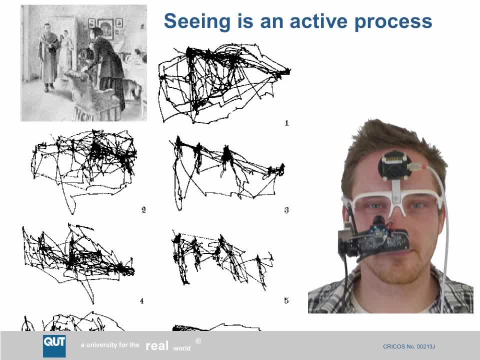 and for that I apologise. And what they did is they take some subjects and they put a device on their head that records the direction in which they're looking, And in these experiments they put this gadget on the person. they show them the picture. 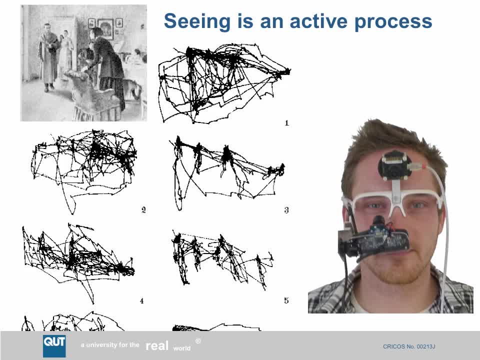 and then they ask some questions, And what's interesting is the direction that the person's eye is looking depends on the questions being asked. So if you ask the person a question like how many people are there in this picture, then what you'll see is a trace where 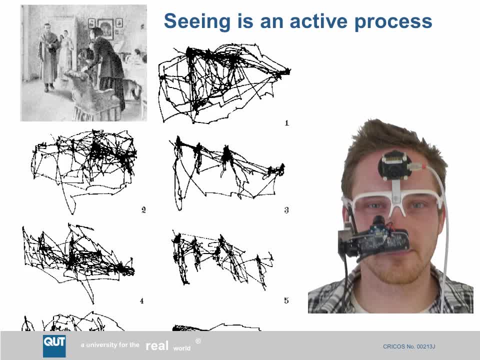 the person's eye is probably just going to go and count heads. It's going to go and look at the people in the doorway- the guy coming out of the door and the lady in the chair, So you can answer the question. Then maybe you want to say: 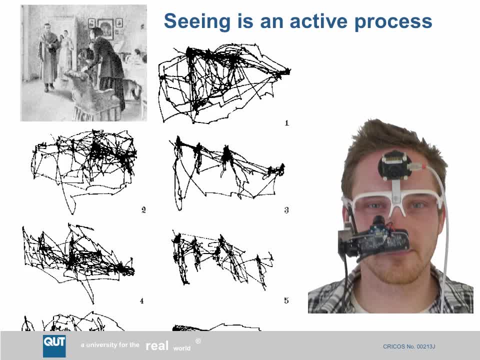 what is that person wearing? How many men or how many women are there? Depending on the sorts of questions that you ask, your eye will take a different path through the scene. So this is really important to understand that seeing is a very active process. 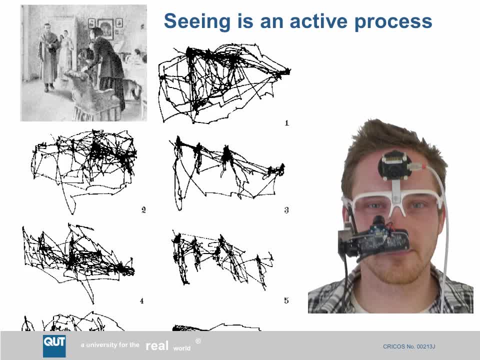 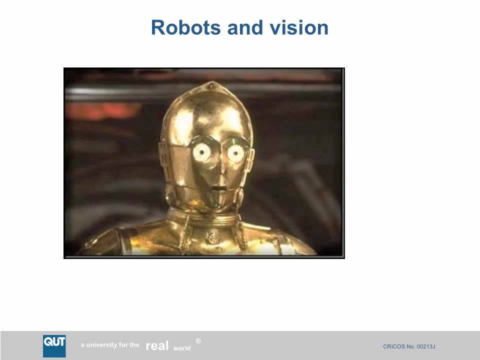 It's also an unconscious process. It's very hard for us to control the direction in which we're looking. Our eye is continually looking everywhere, building up this internal composite model of the world. Okay, ENB339 is all about robots and this particular half of the unit. 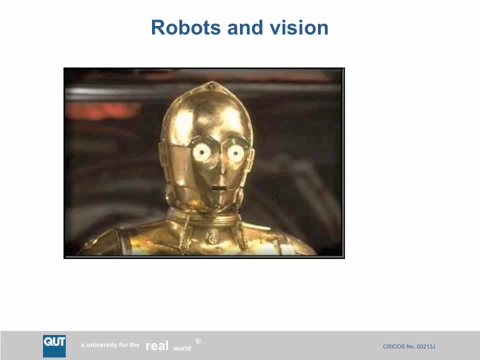 is about robots and vision. So we've seen in Hollywood that robots have vision. Here's a very famous robot: He's got eyes, He's got vision, He can see things and acts a bit like a human being does. That's Hollywood. 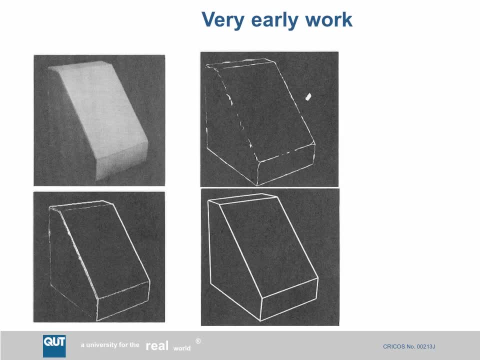 What about for real? Well, in the very early days, in the 60s and 70s, people started to connect computers to cameras, to TV cameras, and try to understand things, images that they could see with the cameras. This is very early work from a PhD thesis in MIT. 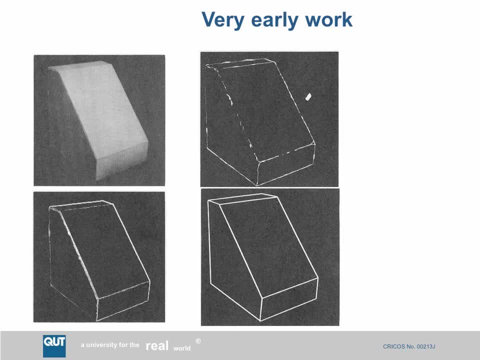 They took a picture of an object. It's not a particularly good representation of the image here, but anyway. they took a picture of the object and then they looked for edges. They look for edges in this image and wherever there's a physical edge on an object. 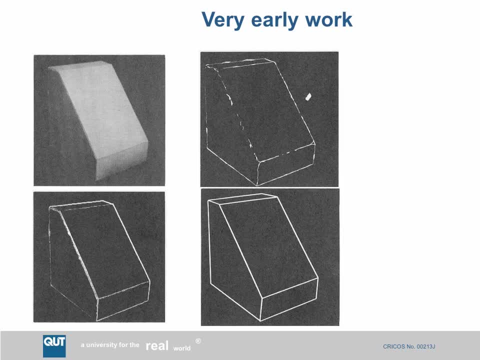 there tends to be a bit of a discontinuity in the intensity. Perhaps there's a shadow, Perhaps there's just an occlusion boundary, where you have one surface suddenly joins a different surface, where the foreground suddenly changes to the background. So if we look for where there are discontinuities, 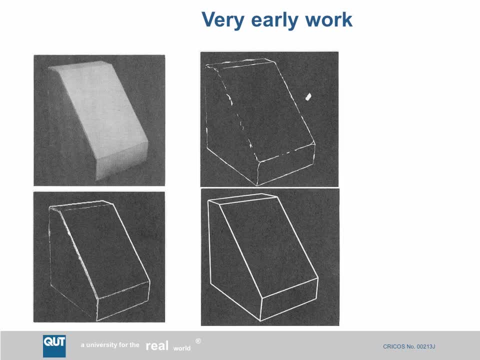 in brightness. we get the image in the top right which is a bit indicative of edges in the world, And then we can apply some computer algorithms to perhaps try and straighten up those edges, to make the edges more continuous, So where there are gaps, 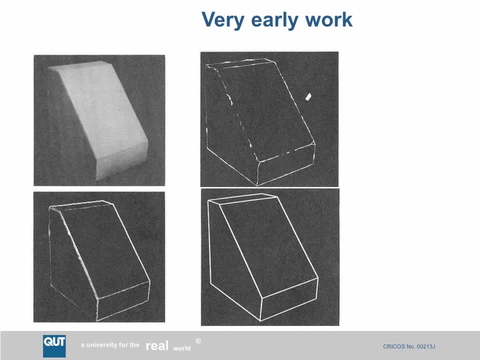 we try and eliminate those gaps. Where the edges look a little bit wonky, we try and make them straight. We end up then with an image in the bottom right corner which is a simple line drawing representation of that original object in the world. 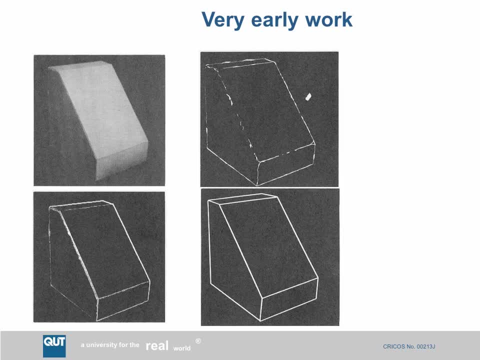 So we've taken an image with a camera and we've converted it into a picture of a nice clean, crisp line representation. So from that then we could perhaps estimate something about the three-dimensional structure of that original object. Very, very early work. 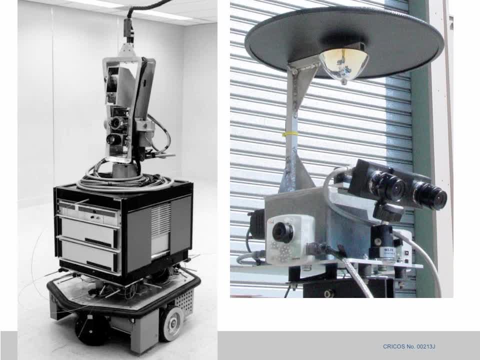 The robot on the left in this image was built at Stanford University in the 1970s- quite a famous robot called Shakey- and has got a number of cameras on the turret on top there. At that time it was very, very slow. 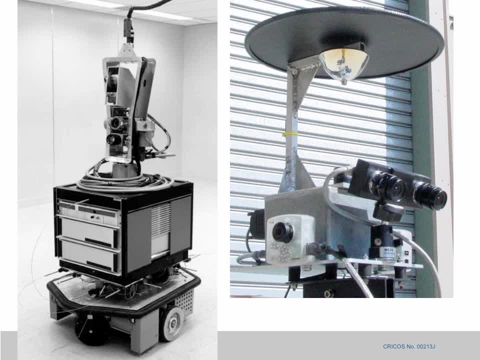 to process images that came from those cameras, but nevertheless, you could use those cameras to recognize objects and to use those to navigate its way around the world Very, very slowly, because the computing power available to this robot Shakey was very, very limited. 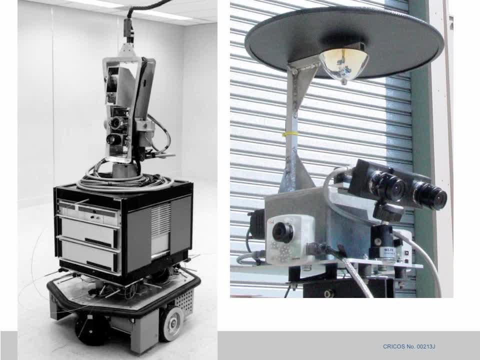 The picture on the right is a bunch of cameras on a robot that I built at CSIRO when I was there probably five or six years ago. There's actually quite a number of different sorts of cameras there, and they're all a bit interesting. 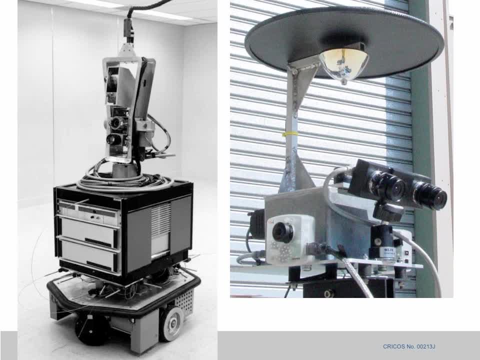 In the front we see two cameras and they mimic a bit the human eye. We have two eyes in the front of our head, so we have two cameras here looking towards the right and we call this a stereo camera pair. And with two cameras in a configuration like that. 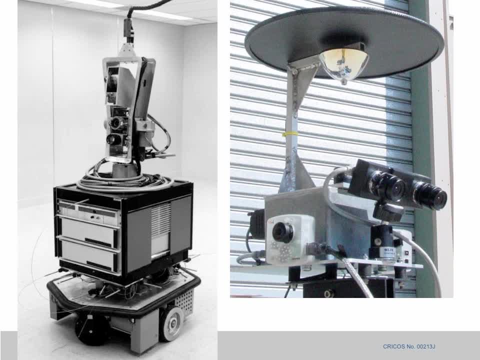 we can work out not just the shape of objects and their color, but we can also work out their size and how far away they are from the camera, And we'll talk about stereo vision in a future lecture. The camera in the plastic case on the bottom left. 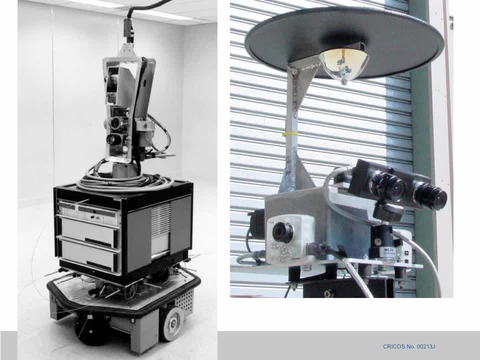 is a fisheye lens camera, So this has got a very wide angle field of view. We can see almost 180 degrees, a whole hemisphere, And that's very useful for a camera that has to perhaps look for obstacles that might be coming from any one. 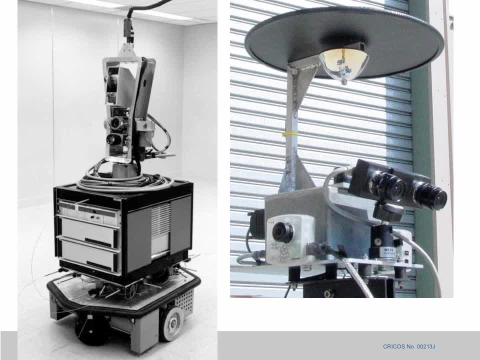 of a large number of directions. Above those cameras you can see a black circular disc and below that you can see a shiny object And that's a mirror. It's shaped a bit like a paraboloid. It's not exactly a paraboloid. 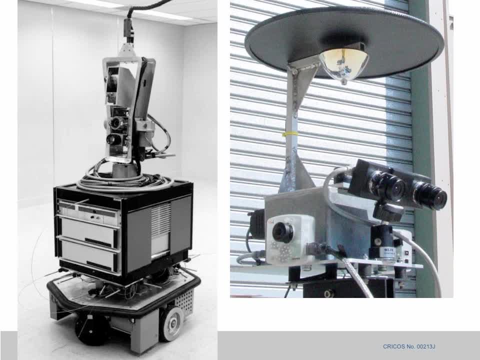 but you can think of it as a paraboloid, And looking up at that is another camera a little bit hard to see behind the stereo camera. So that camera is looking up to the parabolic mirror which then reflects those light rays so that it can see outwards. 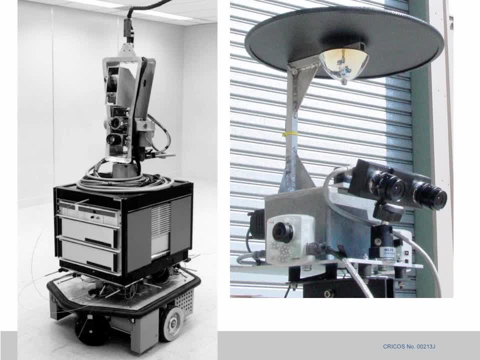 So this is what we call a panoramic camera. It can see in all directions. It can see forwards, backwards, left and right. Again, that's really useful for a robot to have this very, very large field of view. So this is a robot that's bristling with cameras. 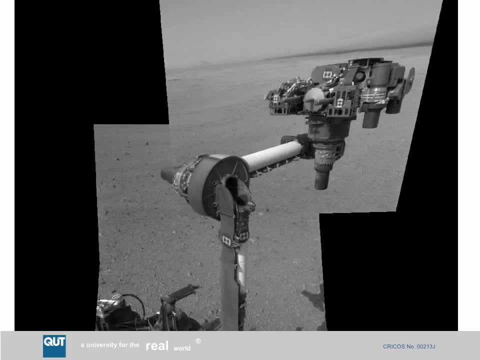 that I built when I was at CSIRO. Here's another very recent robot that's got a lot of cameras. This is one of the arms of the Curiosity rover. It recently landed on Mars And on its head one of its robot arms. 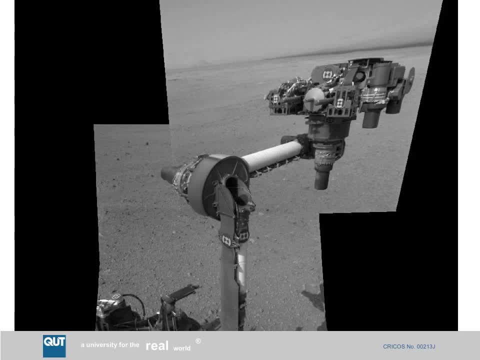 it has a large number of cameras. You can also see a large number of quite distinctive markings. These are optical targets and they're used by cameras to work out the relative position of other parts of the robots, And we'll talk about that a little bit further down the track as well. 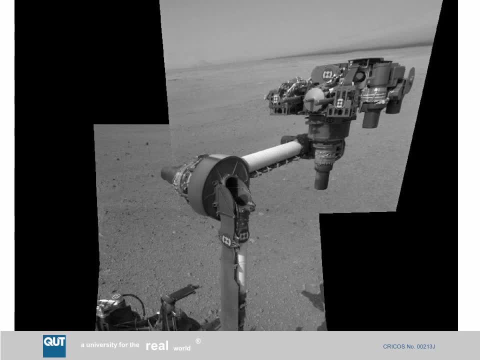 So here are some of the calibration marks. These are very distinctive patterns that it's easy for a computer to recognize this particular pattern in the image and they can use that then to work out the exact position of the robot arm. So vision, I believe. 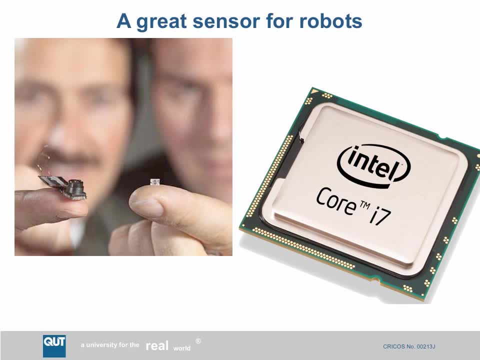 is a really, really great sensor for robots. I hope I've convinced you that vision is a really useful sensor for animals and I think then it follows that it should be a very, very useful sensor for robots. But there are some technological reasons too. 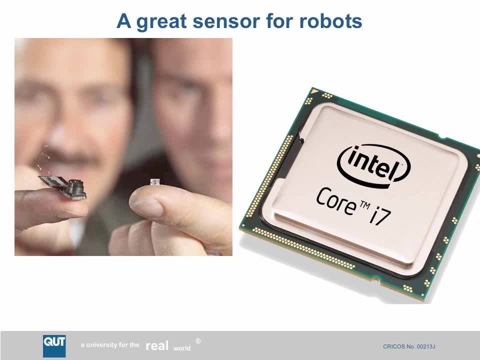 why it's a great sensor for robots. One is: the cameras now are incredibly cheap, and partly this is driven by advances in cell phones, laptops, tablet computers and so on. All of these devices now have got one or two cameras built into them. 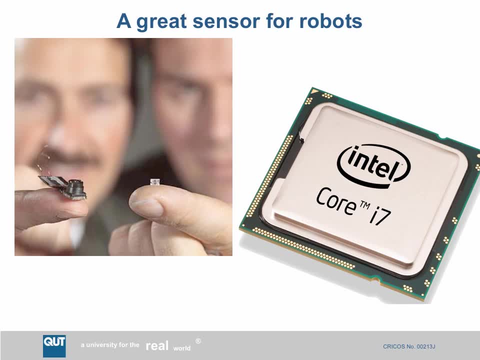 So in bulk, if you're buying quantities of hundreds of thousands of cameras, their cost is less than a dollar each, So that makes them very, very affordable. The other thing that we have going our way is that we have really really powerful computers these days. 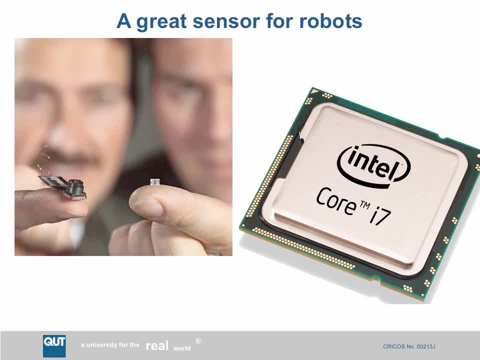 So we can process all of the information that comes out of the cameras and from that information try and work out, create, if you like, a model of the world around the robot, so that we can then do our planning and action. So I'm very, very optimistic about vision. 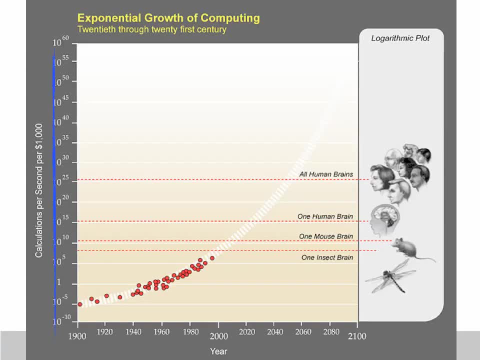 as a sensor for robots. today, Here's an interesting graph put together by a guy called Ray Kurzweil, who's written a number of books about what he calls exponential growth of computing. You can do Google for Ray Kurzweil. 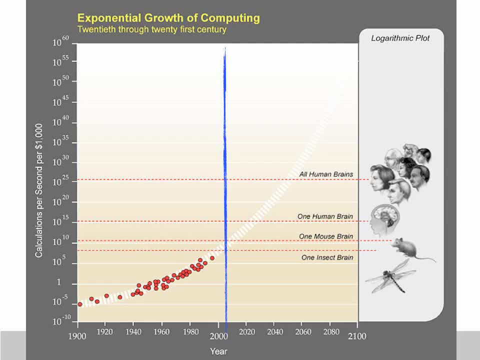 and you'll find a lot of his publications. but what he's done here is he has plotted the number of calculations per second that you can buy for $1,000, and that's this white parabola-shaped curve, And he's taken data points. 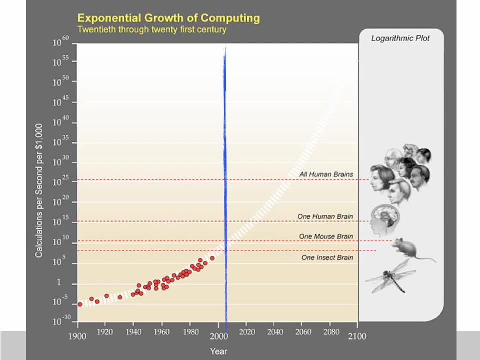 from lots of computers that you could buy, and we can see that he's done some reasonable job of curve fitting here Now. he's also then figured out the equivalent computational power of an insect brain, a mouse brain, a human brain and so on. 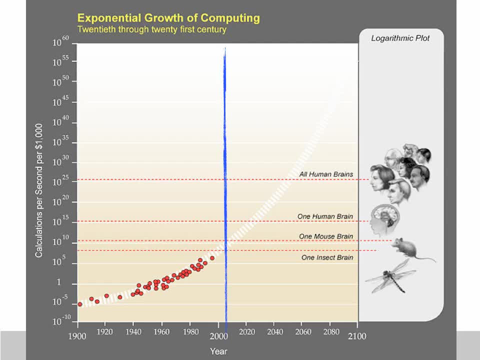 Now, quite how he gets the dollar into insect brain, mouse brain and human brain figure, I don't really know. But anyway, if you believe what Ray says, you look at this curve and you can see that the computational power that's available to us now 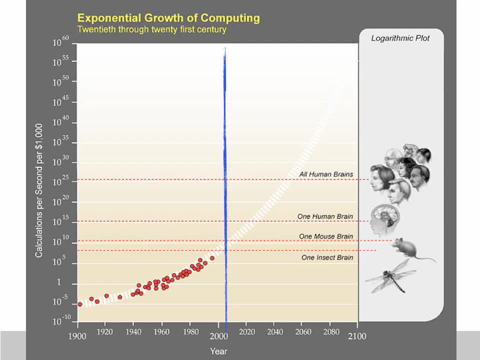 has already exceeded that of a single insect brain and that not very far from now, our computers will have the computational equivalence of a mouse brain And that perhaps by 2020, 2025, we will have the computational equivalent of a human brain. 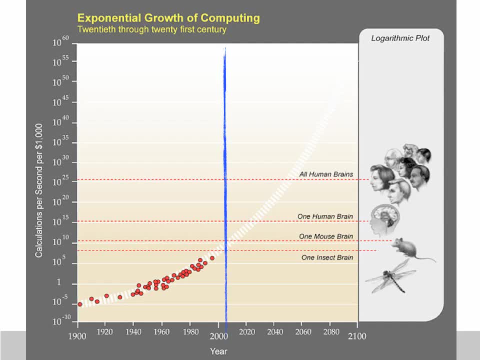 And this is really interesting because that is going to be during your working lifetime- And that by the year- perhaps 2050, 2060, we will have for $1,000 the computational equivalent of all human brains on the planet, And that's just amazing. 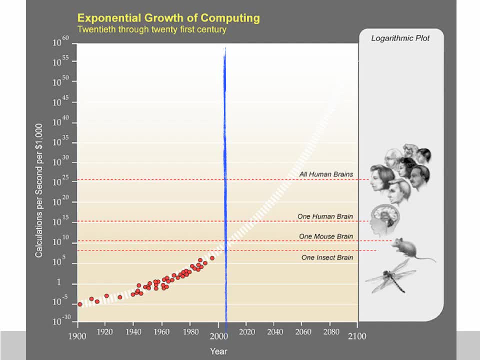 what you might be able to do with that. Again, that's probably certainly within your lifetime, maybe within your working careers as well. So I think there are really exciting times ahead due to phenomenal growth in computing that we've witnessed pretty much in a consistent pattern for 100 years. 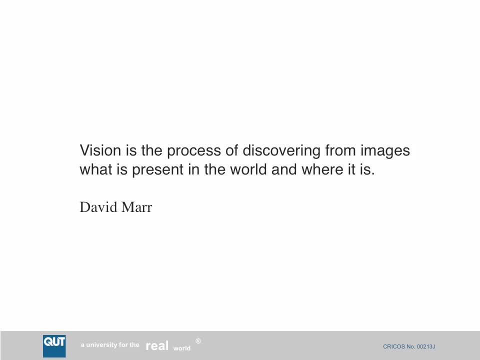 So this is a nice quote by an American research scientist called David Maher who did a lot to try and understand how the human visual process worked and also trying to understand to convert some of those learnings about how the human visual process worked into mathematical models. 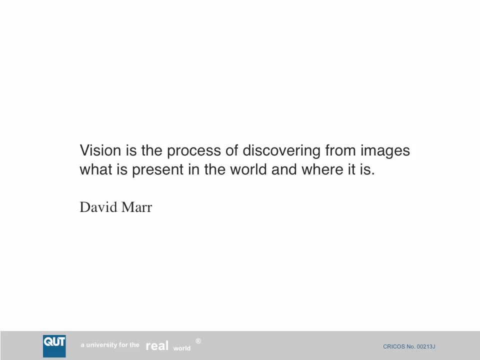 that could be programmed into computers to allow computers to see. So he considers vision as not just a sense. he thinks it's a process of discovering from images what is present in the world and where it is. So I like this idea about it being a process. 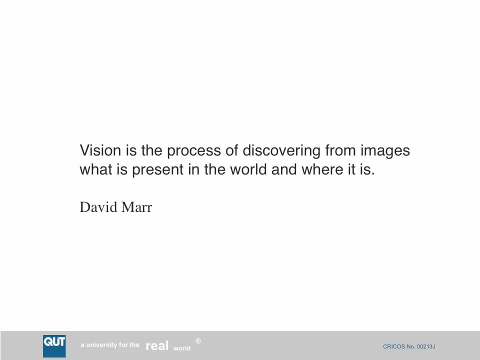 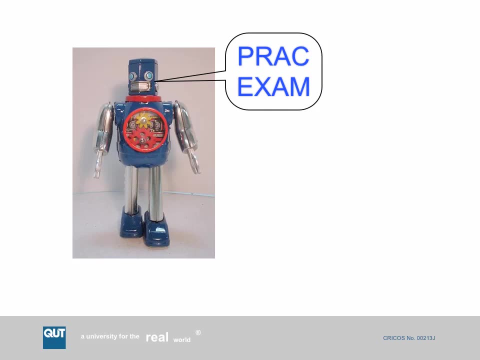 and it being about discovery. Now, some important things to talk about. Now, hopefully, I've convinced you about the importance of vision. I'm going to talk to you about the PRAC exam, which is going to be in week 13.. 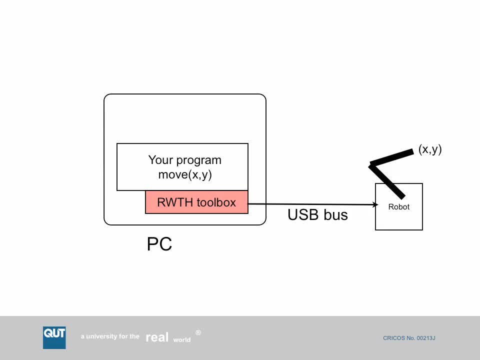 Now so far in B339, you've written some programs in MATLAB on a PC. You've used the RWTH toolbox to communicate with a robot And your task has been to move the tool tip of your robot to a known coordinate or to move it in a straight line. 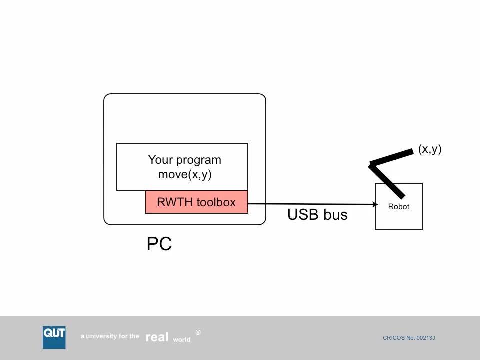 between two known coordinates And you have a PRAC exam on that very, very shortly. So I'm going to assume that this is done, because we're going to build on this for the second part of the unit. What we're going to do. 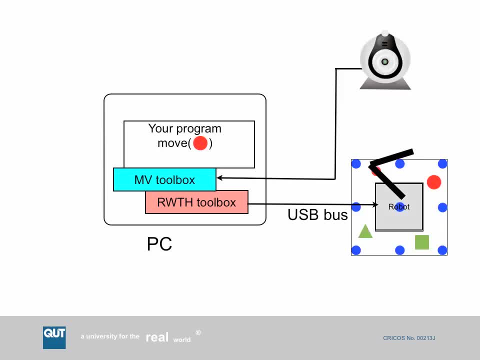 in the second part of the unit is to augment the system. So instead, and what we're going to do is we're going to add a web camera to the computer, and you've probably noticed that all the computers in S or C have 1129.. 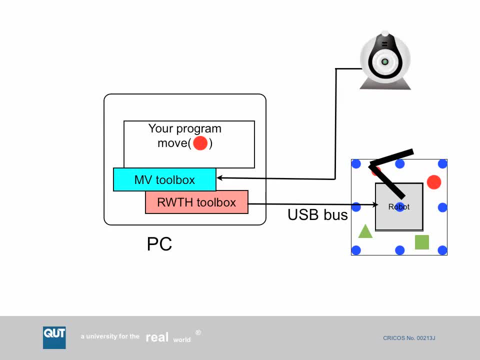 I've got a little webcam on top And you're going to use another MATLAB toolbox- something called the machine vision toolbox for MATLAB, which I wrote and hopefully you have on your USB stick, And you're going to integrate that into your existing robot program. 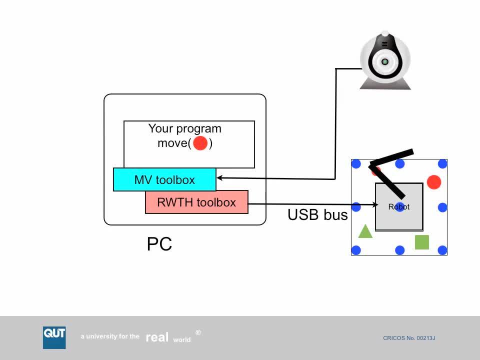 And for the PRAC exam for this part of the unit. instead of giving you a question like move to coordinate, I'm going to give you a challenge like move to the red circle, and I'm going to give you a worksheet. You're not going to see the worksheet. 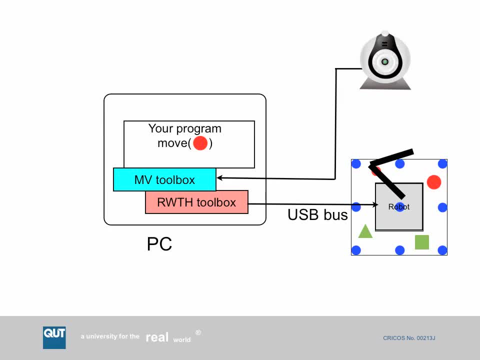 until the day of the PRAC exam. You'll see things like the final worksheet, but you'll have a special worksheet for the PRAC exam. So in order to move to the location of the red circle, you need to solve quite a few problems. 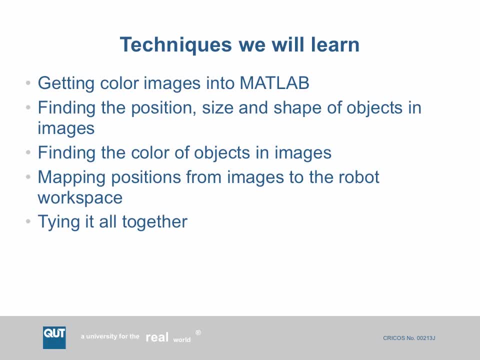 So what we will do is we'll learn about how you get a color image from the web camera into MATLAB. We'll learn how you find the position and the size and the shape and the color of different objects within the image. So that's an important part of the problem. 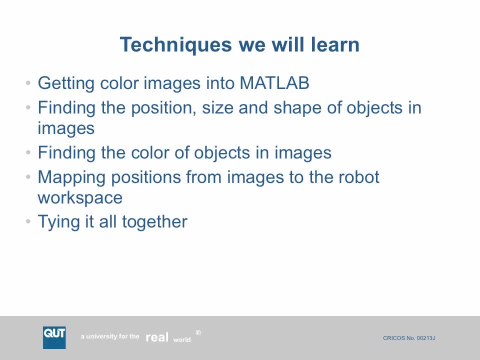 We're going to look at the scene with our camera. We're going to see that there are lots of colored objects there. We're going to be able to work out which ones are red and which ones are blue, which ones are large, which ones are small. 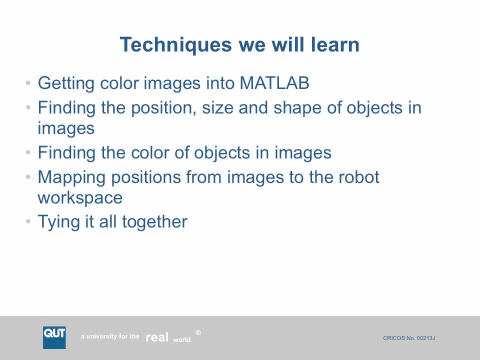 which ones are triangles or circles or squares. The next problem, then, we have to work on is how do we convert the positions of things seen by the camera to the positions of things which can be reached by the robot. The robot and the camera have got different coordinate systems. 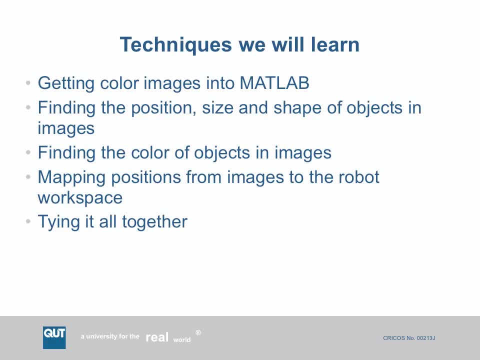 but they're related, So we have to do some work on how we relate those two coordinate systems. These are all techniques that we will learn through the remainder of 3.3.9.. In the pracs, what you'll be doing is tying together the theory. 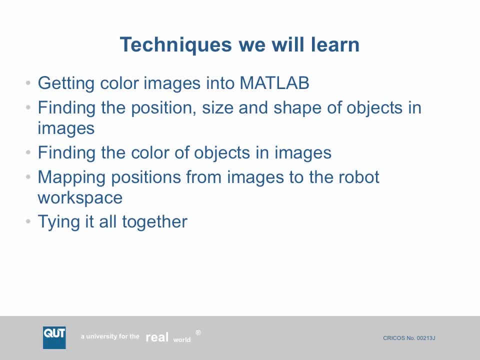 that we learn in class, integrating it into your robot and aiming for that prac exam. So keep in mind that's the end goal. We'll break it down into small numbers, into smaller chunks, week by week, what the goal should be for the prac that week. 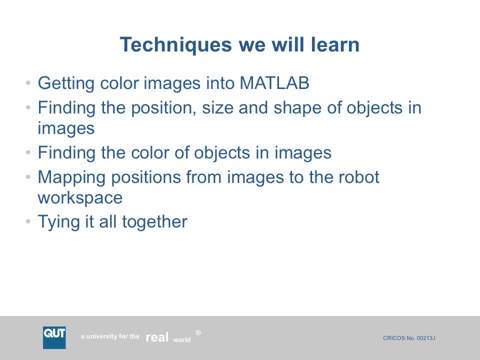 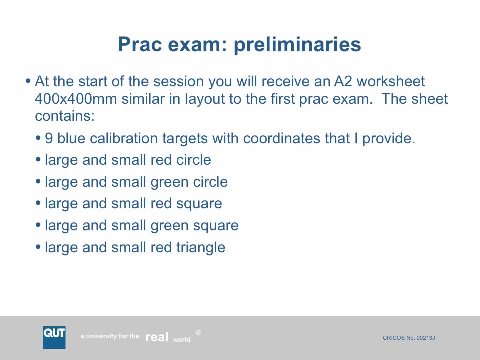 We'll also be using the tutorials to reinforce some of the ideas that we cover in lectures. So the prac exam basically is, as I mentioned before: you get an A2 worksheet, You put that underneath your robot and the sheet contains a number of calibration targets. 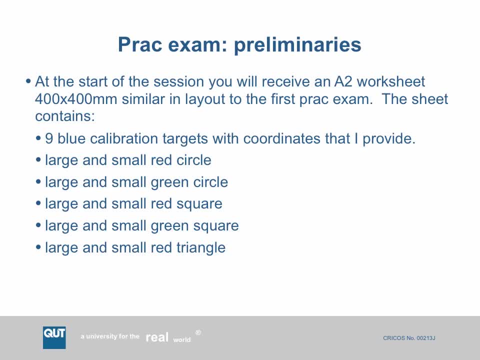 that are blue and some of them have got coordinates. I'll tell you the coordinates of the blue guys, but there are also large and small red circles, large and small green circles, red squares, green squares and triangles, And I'm not going to tell you. 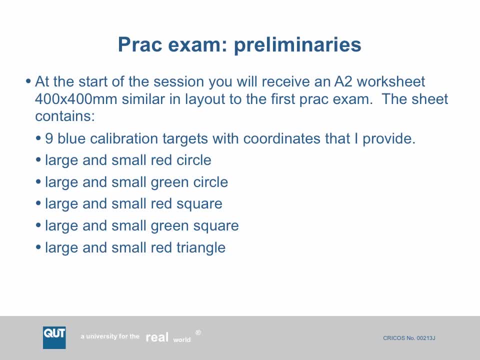 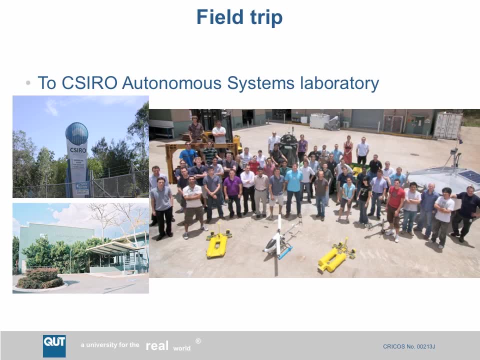 the coordinates of those. You're going to use the camera to tell you the coordinates of those things. The other thing that's really important to talk about is the field trip, And I mentioned this in lecture number one. What I'd like to do- 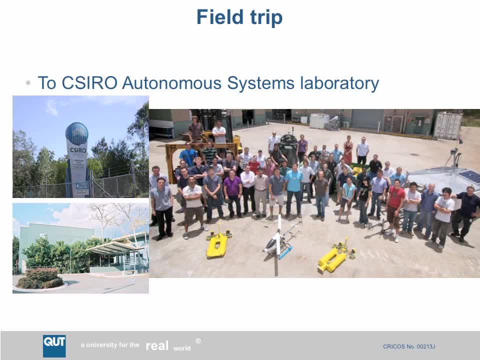 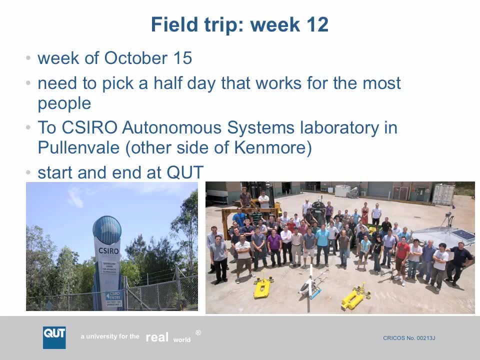 is to organize a field trip to the CSIRO Autonomous Systems Lab later in the it's. I'm down here. Yes, in week 12 or the week of October 15.. So what we need to do is to pick a half day. 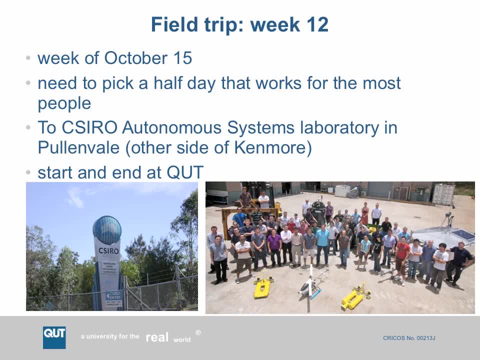 that works for the most number of people. All right, The lab is in Pullen Vale on the other side of Kenmore, and the field trip will start and end at QUT, So we'll organize buses. We'll take you from Gardens Point. 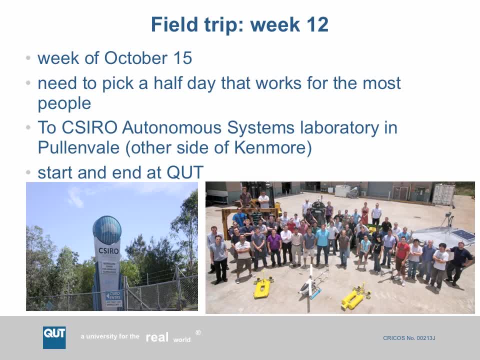 to CSIRO, show you the sites at CSIRO, get to see the labs, get to see some robots, and then we'll go and bring you back again Now. I think to be useful it really needs to be a full half day. I know all of you. 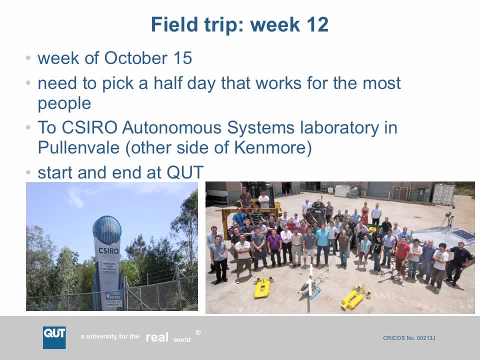 have got different kinds of commitments and it's not going to be possible to find a half day that works for everybody. For that I apologize in advance. So what we need to do is to find a half day that works for the most number of people. 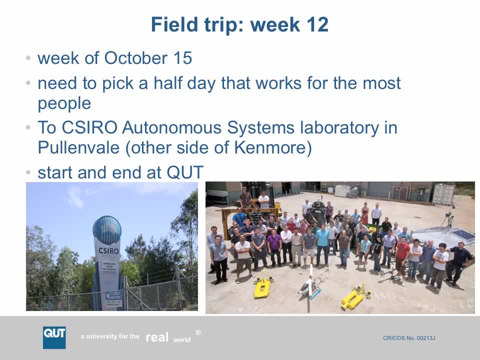 There's nothing accessible about this trip. It's really just for interest and for education. So what I'd like you to do now is to have a bit of a discussion and a show of hands and to pick a half day in the week of October 15. 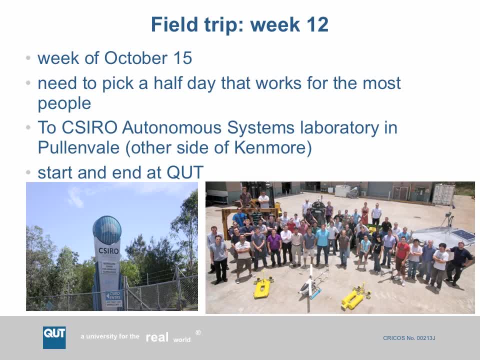 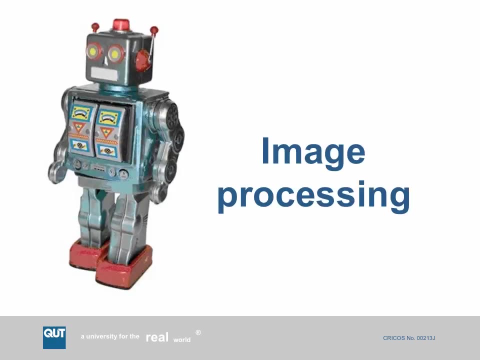 that works for the most number of people, and then I'll organize it with the CSIRO people. So have that conversation and then we will continue. Okay, What I'd like to do in the remaining part of this lecture is just give a quick introduction. 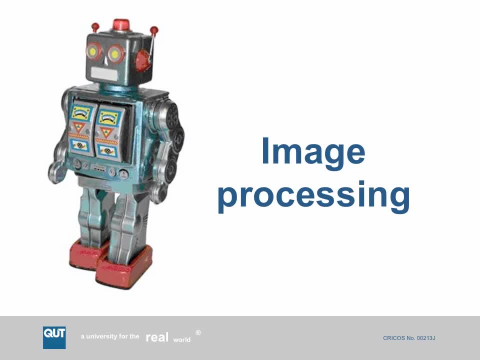 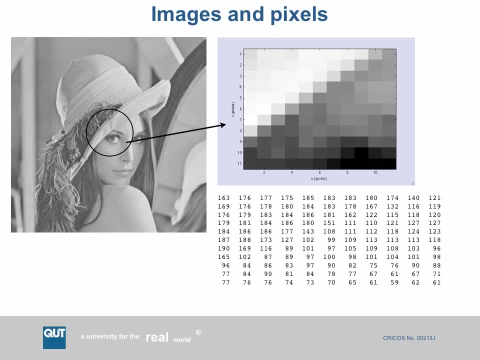 to image processing and particular image processing in MATLAB. All right, Let's get going. If we consider a digital image, it comprises a large number of what we call pixels. Pixel is simply a contraction of picture element, So it's an element of a picture. 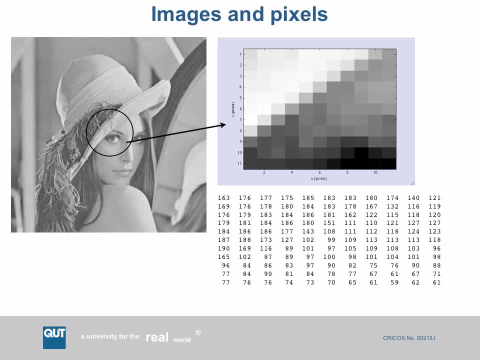 It's the smallest, indivisible element of a picture. So if we zoom in on this picture around the lady's eye, we will find that we can see each pixel as a larger and larger square. We refer to this as being pixelated, If we zoom right in. 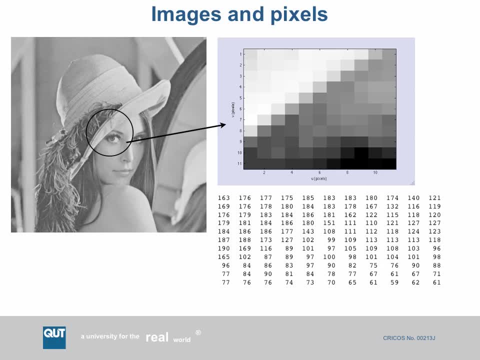 we see that there are some white pixels as part of her eye- the schlera actually, and the darker skin around the eye. If we look at those instead of graphically, like I've done here, if we look at it as a bunch of numbers. 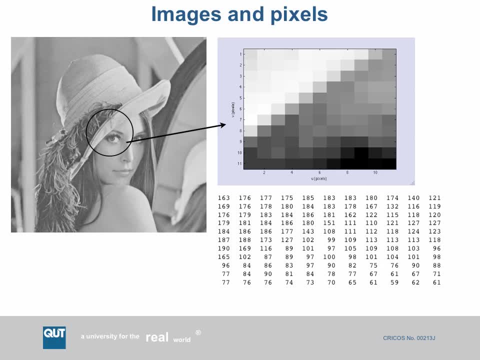 we'll see that the white parts of the image have got big numbers, The dark parts of the image have got smaller numbers And, in fact, the way most images are encoded: a value of 0 means black and a value of 255 means white. 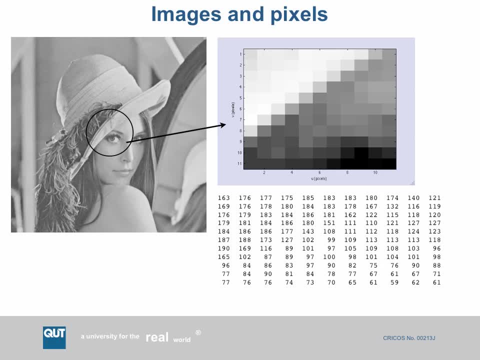 The reason for this is that each pixel is represented by an 8-bit unsigned integer number. So with 8 bits, the smallest number is 0. the largest number is 255.. This is for a black and white image. Colour images are a little bit more complicated. 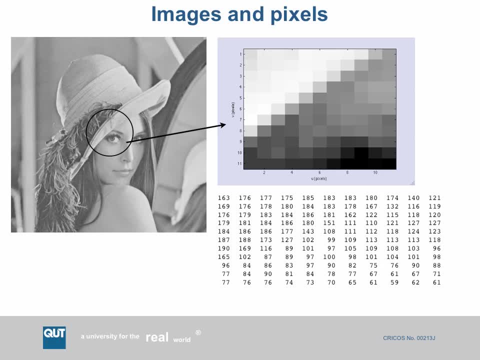 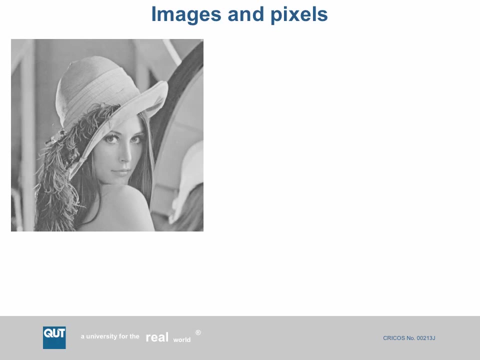 and we'll talk about them in a future lecture, But for right now, we're going to just talk about black and white, or what is more correctly referred to as a grey scale image, where all the colours are shades of grey. OK, if we imported this image into MATLAB. 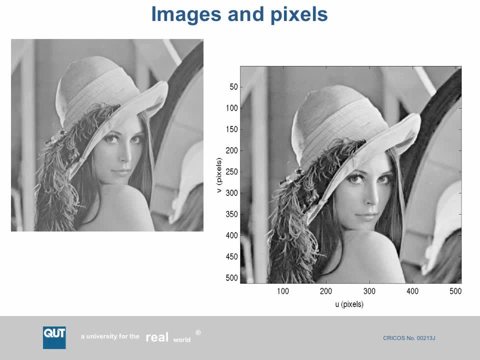 and displayed it. using some of the tools that I'll talk about shortly, we can plot it as an image and we have an interesting coordinate system that's used in image processing. that's a little bit unintuitive and different perhaps to what you're familiar with. 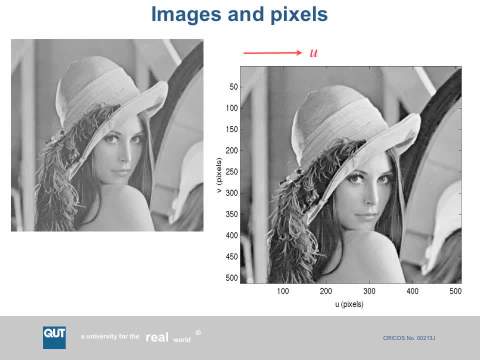 Generally we refer to the U coordinate as the horizontal axis and we refer to the V coordinate as the vertical axis. But what's interesting is that the V axis comes downward from the top corner, So the coordinate is in the top left of the image and the 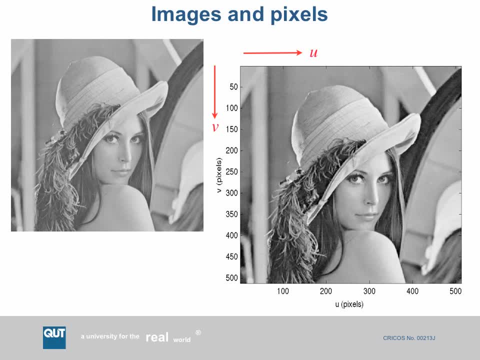 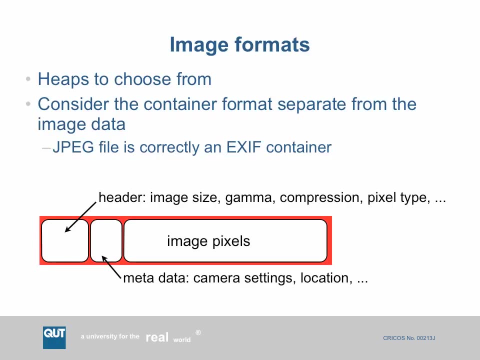 vertical coordinate increases as we move down the image, not up the image as in a more traditional sort of graph. Now you've probably got a directory, many, many folders full of images on your computer, on your laptop, on your phone, on your tablet. Images can be kept. 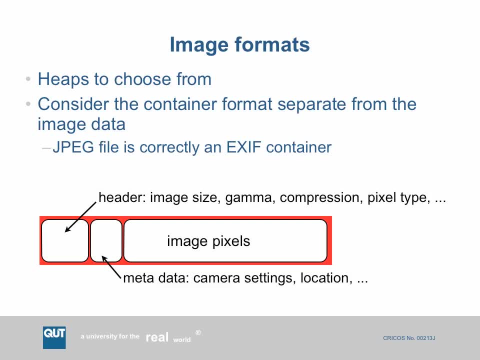 in files on your computer and you've probably seen files like tiff and jpeg and whatever. So an image file is perhaps thought of as a container for all of the pixels that comprise the image And jpeg file, a file that has an extension jpg. 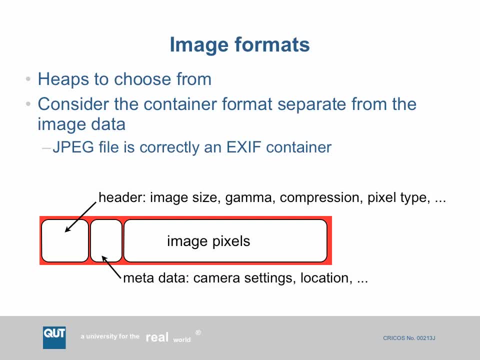 is actually more correctly known as an xif container. So it's a well defined standard container And within that container are different compartments which hold different types of information. So within the container there is a header section which is how big the image is. it talks about how it's being compressed. 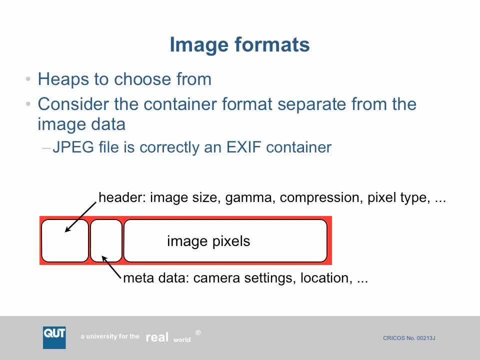 how big the pixels are. Are they 8 bit numbers, Are they 10 bit numbers Or something like that? There's another section called the metadata and that contains information like where the camera was. if your camera's got a GPS, it'll contain the. 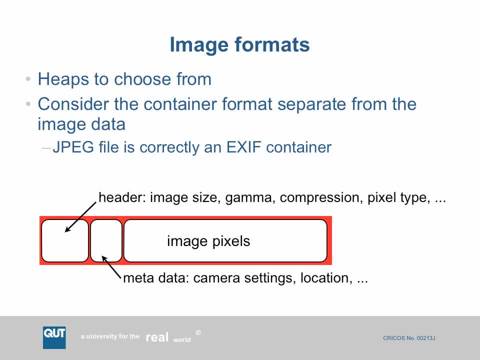 GPS data. It'll contain the time and date at which the picture was taken, the focal length of the lens, whether the flash was used, and so on, And then, finally, there's the part of the container that contains the image pixels. Often times, 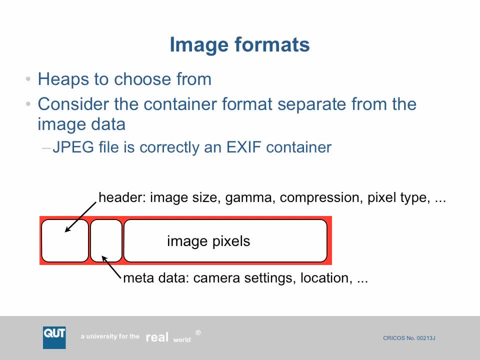 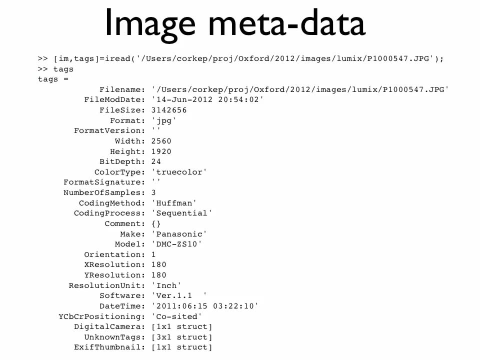 compressed, because images generally have a lot of pixels that take up a lot of room on disk. so there's been a lot of work on image compression to make images smaller. So here's an example of the image metadata and this is a MATLAB command that you could. 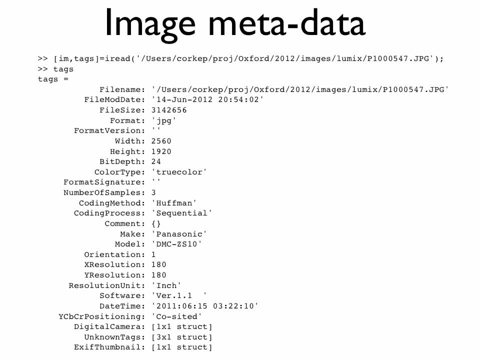 issue with the machine vision toolbox and we see here that there's a lot of data that's recorded with the image. We can see the width and the height, the way it was compressed. we can see something about the make and the model of the camera that took it. We can see 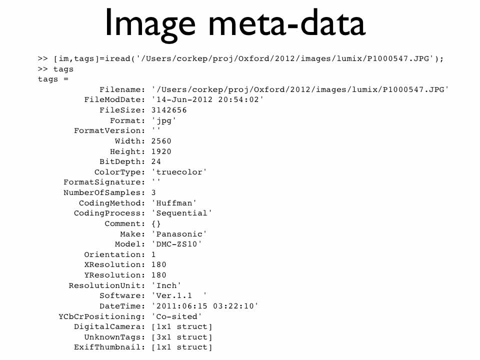 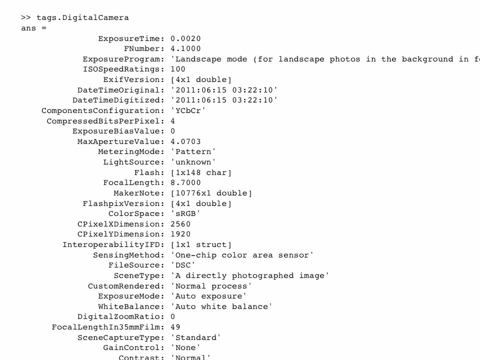 the number of pixels per inch in the sensor. We can see the date and time at which the image was taken. We drill down into that some more. we can see the exposure time, the F number, that the camera was in landscape mode- ie I was holding it horizontally. 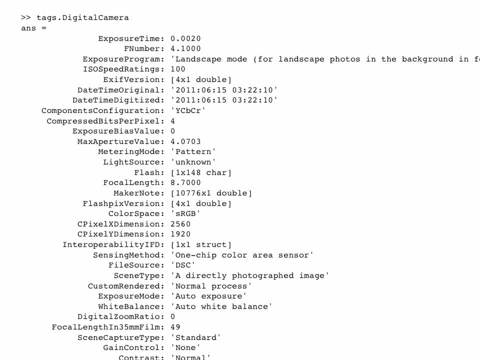 What else can I see? I can see the focal length. I can see the type of colour space that was used. I can see more information about the sensor. There's a huge amount of information associated with an image that isn't what you see. 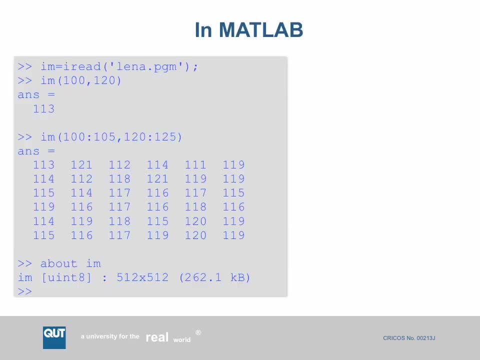 This is referred to as metadata. We talked earlier about the need for image compression. That is, we want to save our images but use as few bytes on the hard disk as possible. There are two forms of compression that are commonly used. one's called lossless. 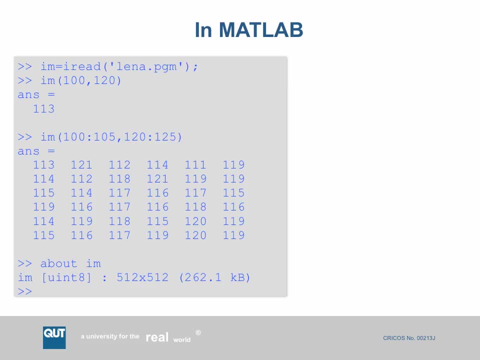 and one's called lossy. Lossless compression exploits redundancy in the image. It's able to squeeze all of that pixel data into fewer bytes on the disk, and then, when it comes to uncompression time, it can restore the original image, and absolutely no data is lost. 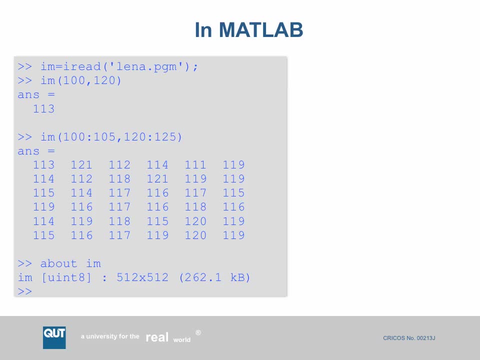 The original image is exactly the same as the image that's been recovered after compression. Now, if you do this lossless kind of compression, there's a limit to how much compression you can get, and typically the best you can do is to reduce an image to about. 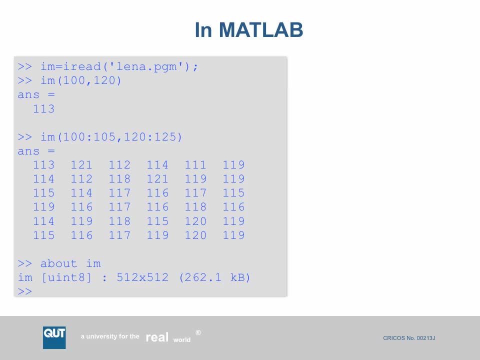 30% of its original size. That's the best you can do with lossless compression. The other option is lossy compression, and JPEG is a lossy compression algorithm. What it does is it exploits limitations in the human vision system. The human vision system is not. 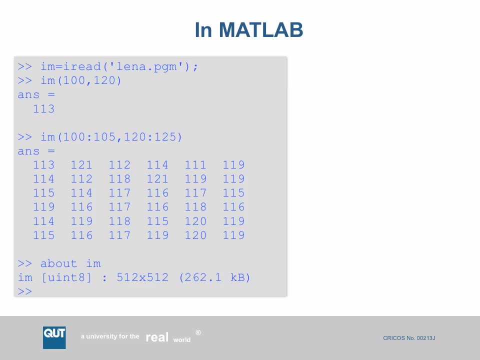 perfect, and far from it. We're actually not very good at noticing very fine detail in images, So we remove that fine detail and that saves bytes. Also, the human vision system is better at determining differences in intensity than it is at determining differences in colours. 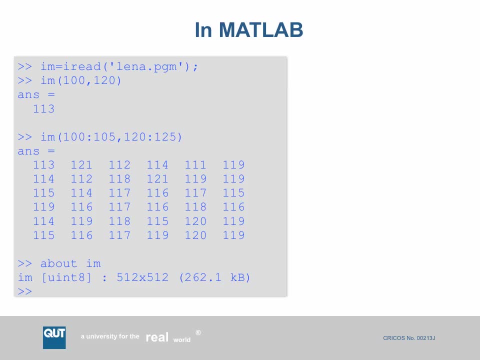 And so lossy compression also exploits this. It tends to make colours more similar than they really are, because the human eye won't detect that that change has been made. So by exploiting these wrinkles in the human vision system, we can reduce the amount of data required to represent the image. 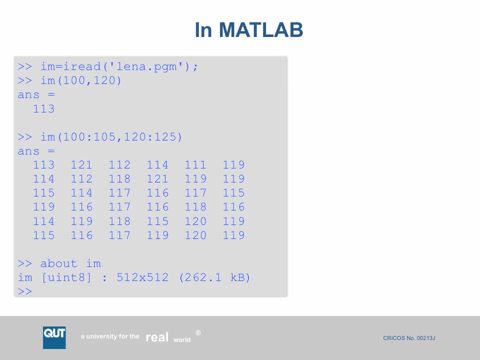 quite significantly. But if I took an original image and then an image which I've compressed and then uncompressed, they'll look the same to a human viewer, but if I look down at the individual values of the pixels they'll be different. So it's important to remember that's a 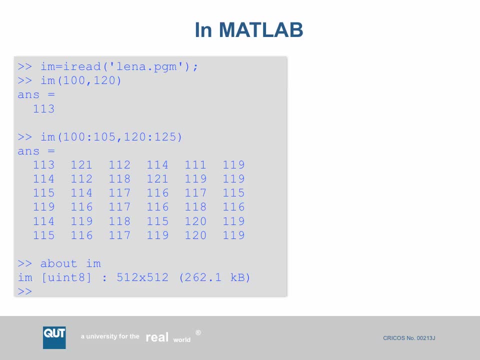 characteristic of lossy compression. Now let's talk about MATLAB, because that's going to be the tool that we're going to use for the prac, and it's also going to be a tool that we're going to be using in tutorials as well, and certainly the tutorial just coming up. 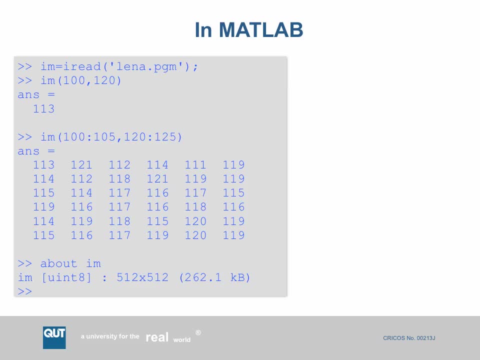 So, using the machine vision toolbox for MATLAB is a function called iread, and in this example, what we do is read an image which lives in a file called linapgm. The lina image is the lady that you saw in a few slides ago. So I read that. 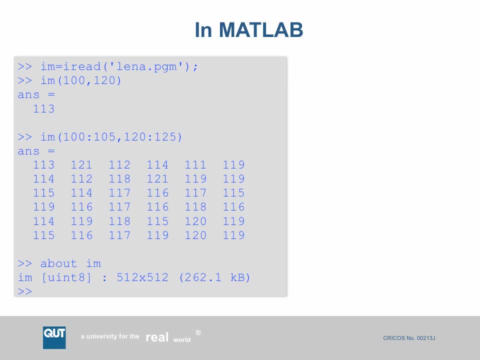 in into a MATLAB variable called im. And now, if we look down the bottom of this list of MATLAB commands, here there's the command about im, And what that says is that im is 512 by 512 matrix and the elements in that matrix are all of the uint8. 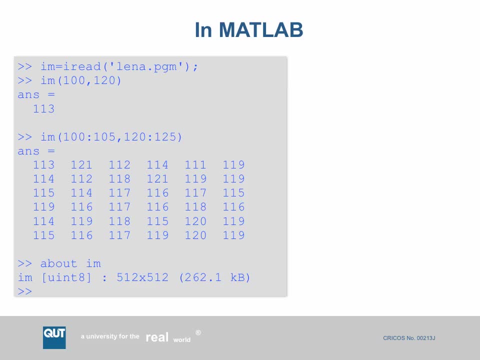 type, That's an unsigned 8 bit integer type. So these are numbers that can only be between 0 and 255, as I mentioned previously. But it's a matrix. It's a 512 by 512 matrix. We can think of it as an image, but we can also think about 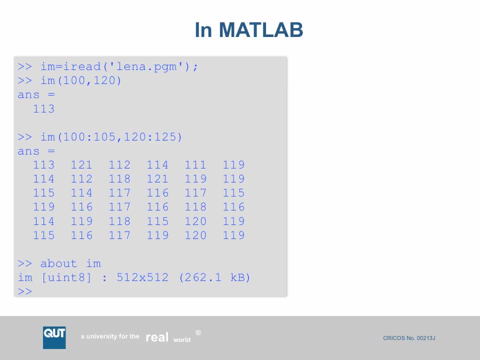 it as a matrix and this is important. So the second command on this page is we look at the value at coordinate 100- 120.. So that's row number 100 in the image, column number 120. so that's, if you like, the vertical coordinate is first. 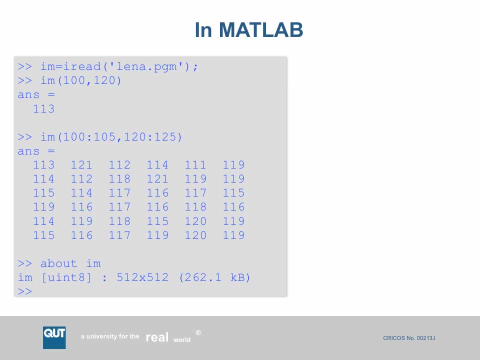 followed by the horizontal coordinate, and we'll talk about this in a moment. Anyway, that particular element in the image, the pixel has got a value of 113.. That's about half way between 0 and 255. so it's kind of a middle grey colour. 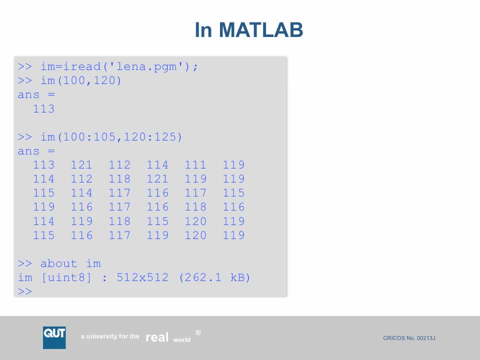 The next command. what I'm doing is using some MATLAB notation to print out the values of a small sub-region of the matrix. So I'm wanting all of the rows between 100 and 105 and all the columns between 120 and 125 and the result. 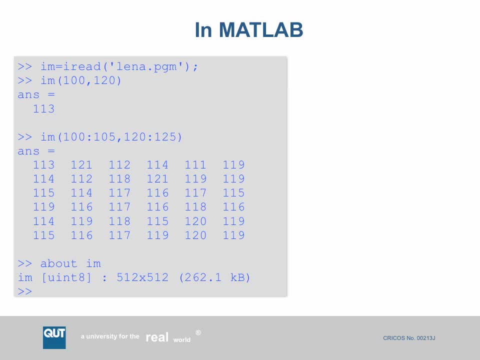 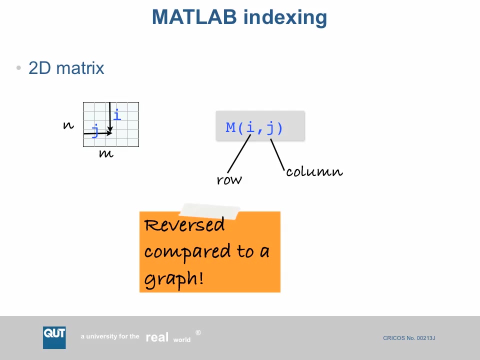 is a 6 by 6 matrix, and what we see in here are the pattern of grey levels in this little tiny 6 by 6 pixel region of the larger Lanner image. I mentioned just a little while ago that we can represent the values of pixels. 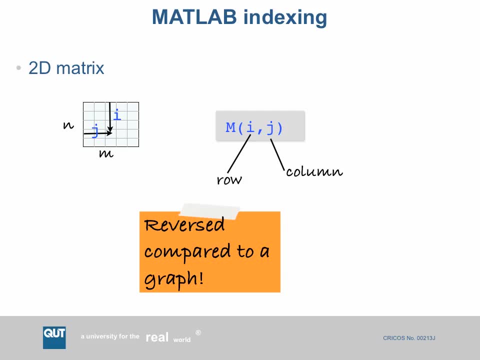 as a number and the example. previously the numbers were in the range 0 to 255. they're represented by an unsigned 8 bit integer. It takes just a single byte of computer memory. In MATLAB it's quite common to represent pixels by double precision numbers. 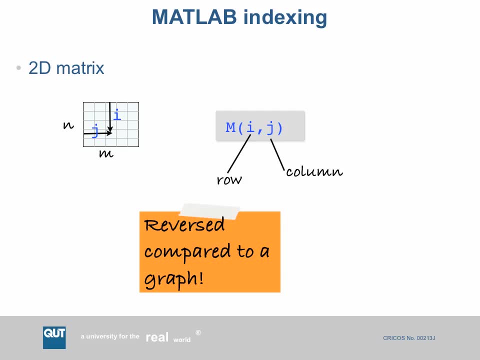 in which case each pixel takes 8 bytes of computer memory. In that case they range. the convention is that they range from 0 to 1, where 0 is black and 1 is white. So what are the advantages of using double precision? 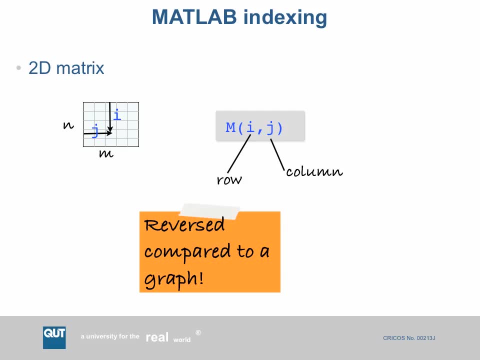 arithmetic with all that extra memory versus using simple single byte representation. One of the problems with integer arithmetic, particularly with very small word sizes, 8 bit numbers, is saturation. So if I add, for example, 100 plus 100 plus 100, 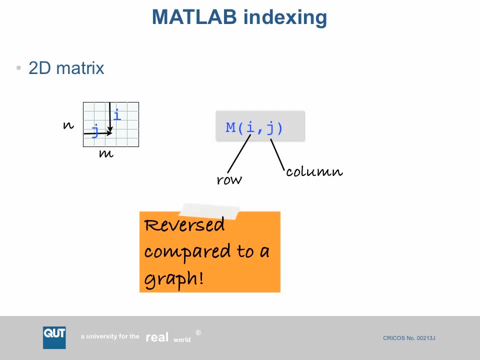 we know the answer should be 300, but in 8 bit arithmetic we can't represent the number 300, it's just too big, and what MATLAB will do is substitute the closest number that it can to 300, in this case only 255. 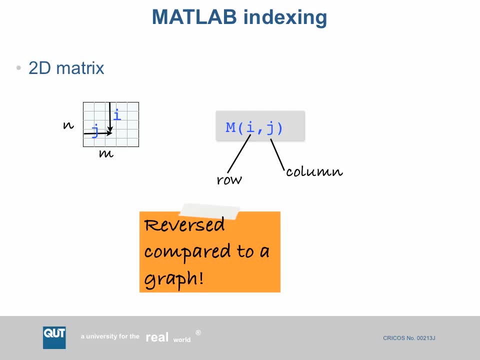 So we get odd effects where things like 100 plus 100 plus 100 becomes equal to 255, and that can cause unexpected problems. If you do it in double precision arithmetic, you don't have any of those issues at all. Another issue with using integer arithmetic is: 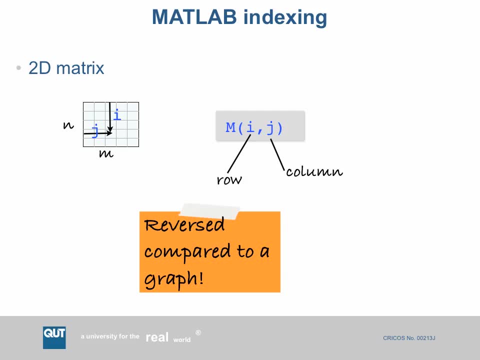 truncation. So in the example shown here, 150 divided by 151, the answer is equal to 0.. Because we can't represent a fraction, and that's just the way it is with integer arithmetic. Again, it's a surprising result. 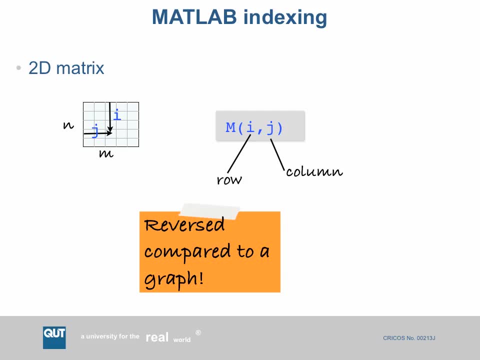 that's an unexpected result, but that's one of the consequences of using short 8 bit representations of numbers. You save on memory, but you pay for that in terms of arithmetic grief. With the MATLAB toolbox, we can convert images from unsigned integers to doubles using the function I double. 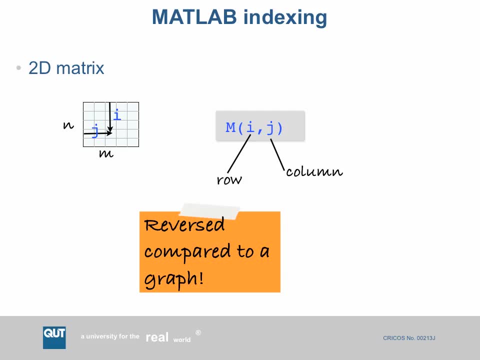 and we can convert them from double representation to integer representation using the function I int. I talked also a couple of slides ago about indexing in MATLAB. If we consider that an image is represented as a matrix, then we need to understand the relationship between the traditional 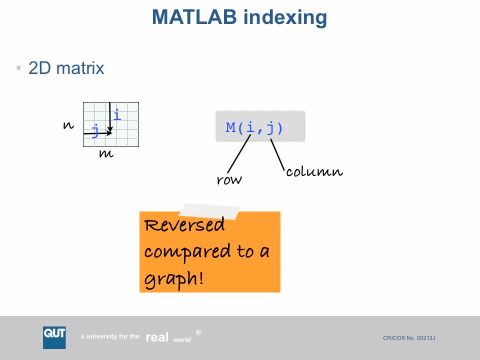 row and column addressing of a matrix. So when we index into a matrix, the first subscript is the row, the second subscript is the column. When we think about it in terms of an image, that means then that the first subscript, the first index, is actually 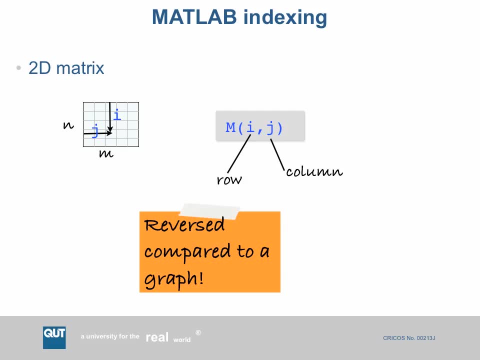 the vertical coordinate. the second one is the horizontal coordinate. So generally when we write the coordinate of a point on a plane, we say where x is the horizontal, y is the vertical. It's reversed, and this can also be a common source of grief to people who 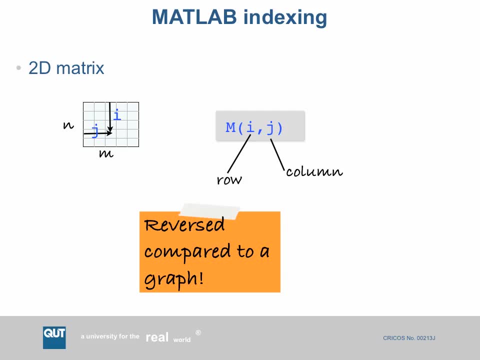 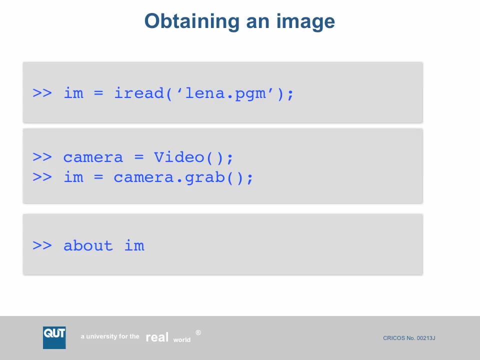 are starting off using MATLAB for image processing. So remember that the indexing convention, when you treat it as a matrix, is flipped. the coordinates are flipped with respect to a traditional planar graph. It's useful also to talk just briefly about MATLAB indexing more generally. So the first line. 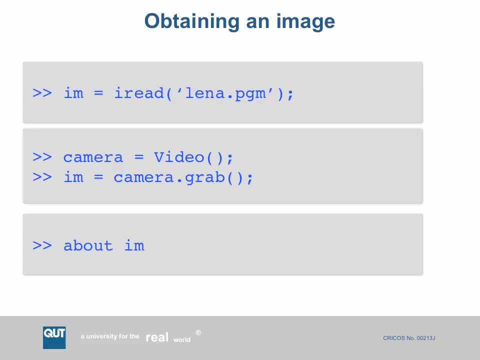 here we create a matrix with 100 rows and 200 columns, and the matrix is filled with random numbers in the range 0 to 1.. The second line then picks out just a single element of that matrix. It picks out the element at row 30 and column 40.. 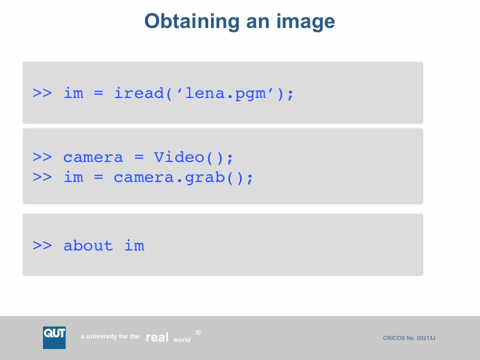 The result is a scalar, a 1 by 1 matrix. The next line is saying: I want to select all the rows between 1 and 100 and column 50. So what that's going to do is to take a vertical slice through this matrix at column. 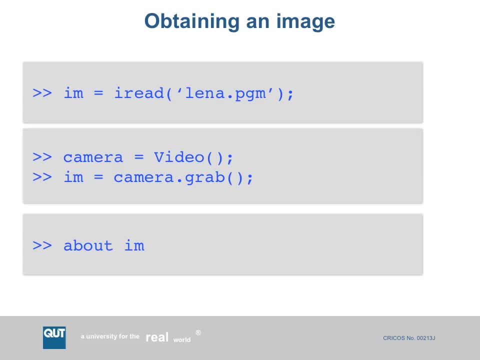 50, from row number 1 through to row number 100.. The next line does something similar. What it's going to do is to take all of the rows from row 1 through to the end. End is a special keyword. that means the maximum possible. 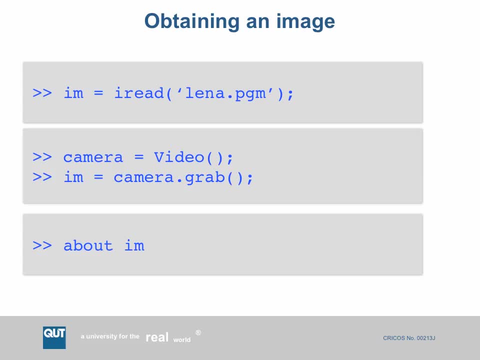 value that that subscript can have, and in column 50.. So what it's going to do is for column 50. it's going to take all the elements from row 1 through to the last row. In this case it's the 100th row. 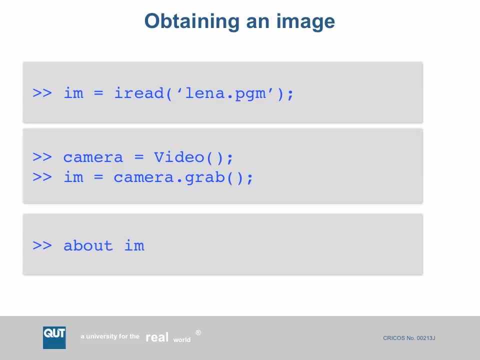 So it's going to take a slice, a thin slice, one element wide, right down through the matrix. The last line after that produces exactly the same result as the line above. So the expression 1 to end, So you can think of the colon operator as being: 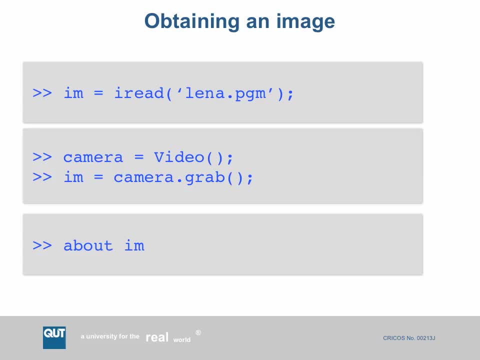 synonymous with the word 2.. So it's the range from 1 to end. We can write that in an abbreviated form and just use the colon alone, So m colon. comma 50 means take column 50 from the matrix or rows within column 50.. 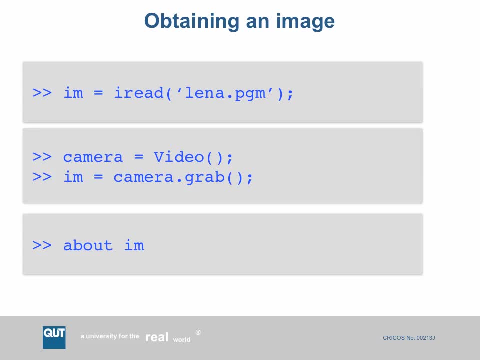 Now we move to chopping out not just a line from the matrix, but chopping out a sub region, an area of the matrix. So this is saying we're going to take the sub region defined by the rows 20 through 30 and the columns 40 through. 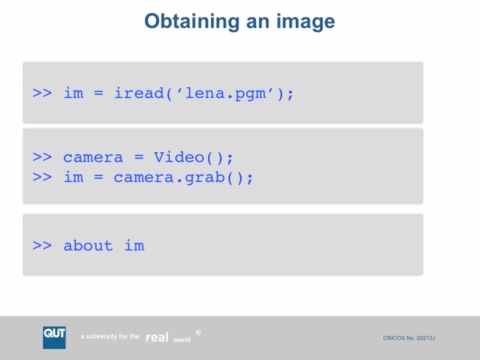 50.. The line after that is doing an interesting thing. What it's going to do is to take the columns in the reverse order, And so what this is saying is: we're going to take all of the rows from row 100 to row 1 in steps of minus. 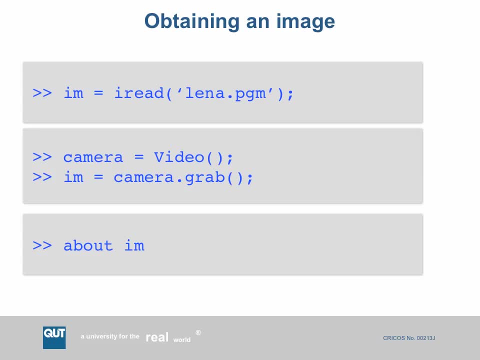 one. So we're going to start at the bottom of the matrix and work our way up And we're going to take all columns. So what that's going to do is to swap the rows of the matrix, So the bottom most row becomes the top, The second. 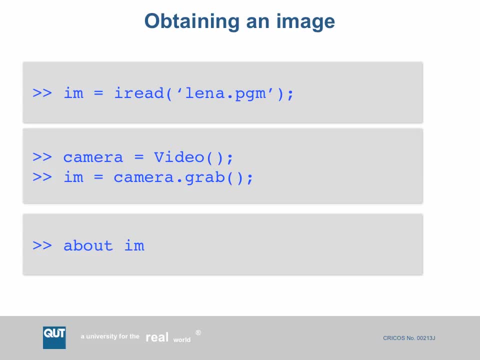 bottom most row becomes the second top. So, if you like, what we have done is flipped the matrix around a horizontal axis. So these are some quite clever tricks that you can do Some quite complicated manipulations on the data using a very concise MATLAB shorthand. 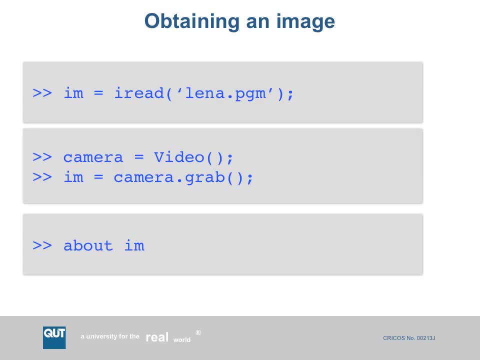 These techniques, these indexing tricks, things that you need to become familiar with. The very last line here is sub sampling the image or the matrix. So what it's saying is starting at row 1 in steps of 5 through to end. So we're going to go row 1,. 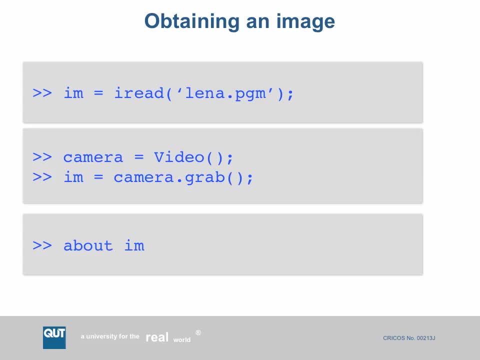 row 6, row 11 and so on, And then for the columns, we're going to take column 1, column 3, column 5, and so on, all the way up to the end. So we're going to end up with a smaller matrix. 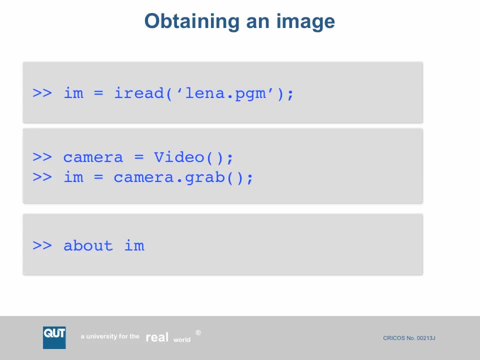 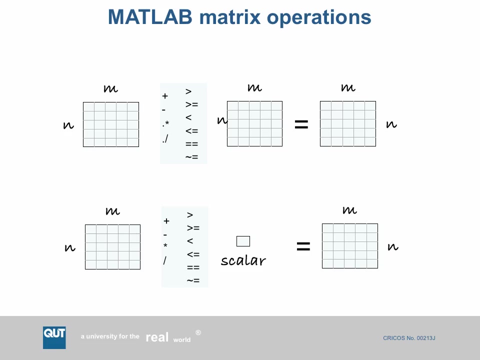 In the vertical direction it will have one fifth the number of rows of the matrix M. In the horizontal direction it will have one half the number of columns that M has. Here's a quick summary or cheat sheet of functions for getting an image into the MATLAB workspace. The function: 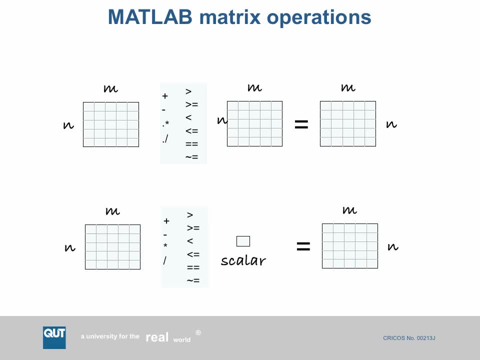 I read we met previously. The argument is the name of a file that contains an image, and the image file is found, The image is read out of it and the workspace variable I M contains a matrix of pixel values that correspond to that particular image. This function's got a large number of 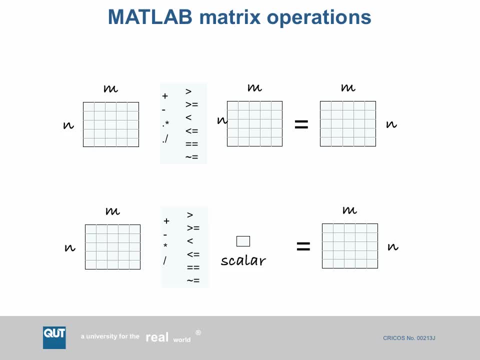 options. so check the help documentation to see what those are. The next group of functions are for grabbing an image from a camera if you've got one attached to your computer. So the function video with a capital V returns not an image but a camera object. 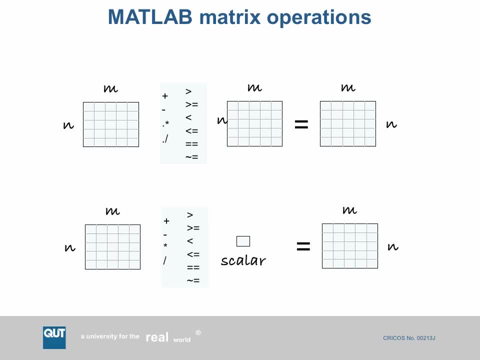 So this variable camera is a special type of MATLAB variable. It's an object. Now that object has got a number of functions associated with it. They're called methods, and one of those methods is called grab. So if we invoke the grab method on the camera object, 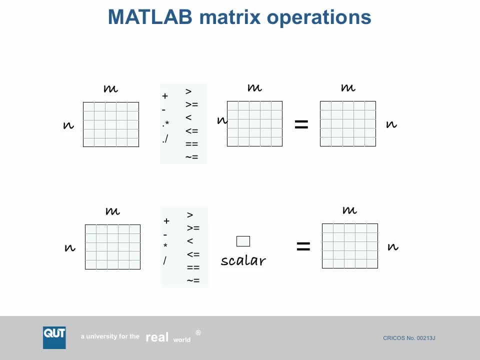 it returns an image, And so that's what the second line does. So the first line you only do once You create a camera object. The second line: you use that camera object to grab an image whenever you need one, And what it'll do is wait for the next. 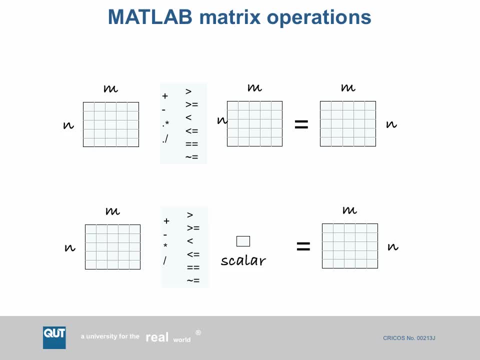 frame to come from the camera. Grab that and place it into the workspace variable im. The function about is just a simple convenience function that tells you some information about a variable, Tell you the number of rows and columns and the type of data that's within. 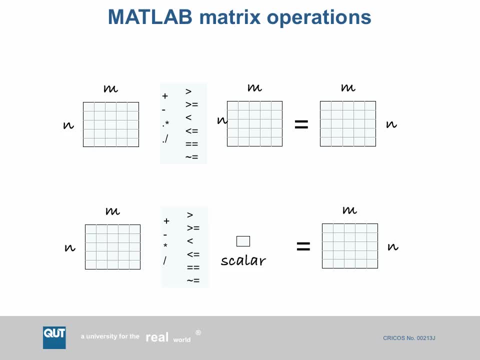 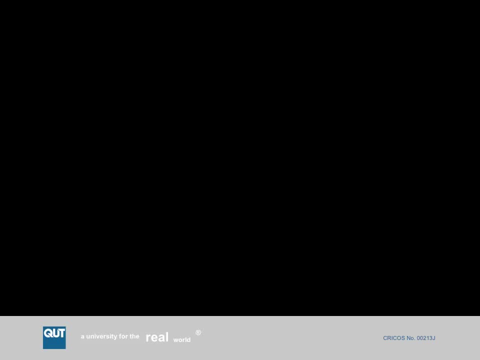 that variable, Whether it's an unsigned integer or a double or whatever. The final set of tricks I want to talk about are MATLAB's matrix operations. MATLAB can do very simple things Like one plus two, and it will tell you the result is three. You can also do: 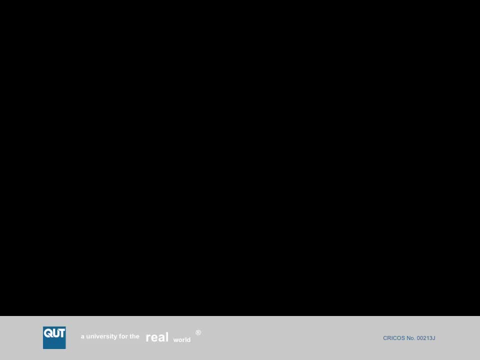 those sorts of arithmetic operations on matrices. But the matrices need to be the same size. So consider, we've got two matrices. Each one has got n rows and m columns. If we add them together, what MATLAB will do is add the corresponding elements of each. 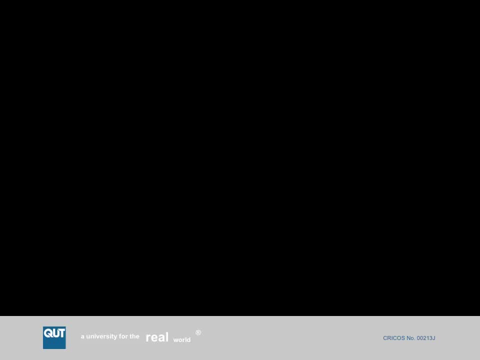 matrix and place them into the corresponding element of the matrix on the right hand side of the equal sign. So we can do element wise addition, subtraction, multiplication and division. So notice, if you want to do element wise multiplication or division, you use an unusual operator. You say: 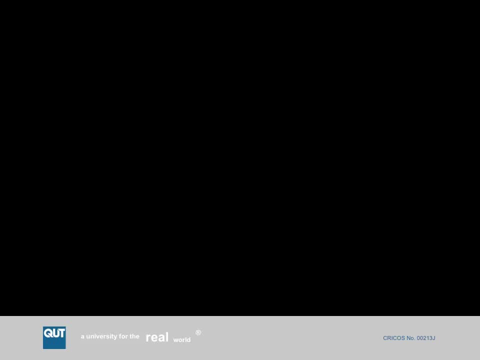 dot star or dot slash. There can be no space between those two symbols, So it's a dot followed by a star or a dot followed by a slash, And that's element wise operation. If you have a matrix star, another matrix, then MATLAB will attempt to do matrix. 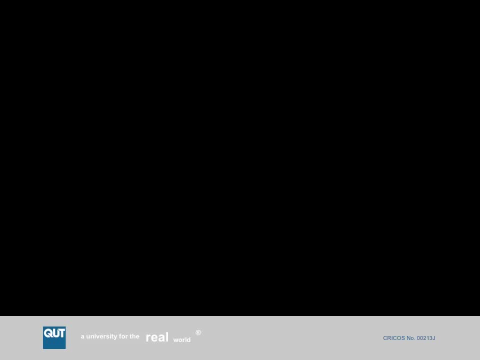 multiplication, Where you take the dot product of each row and each column and assign them to the corresponding element on the right hand side. MATLAB is very good at doing element wise operations as well. Matrices must be the same size In addition to arithmetic. 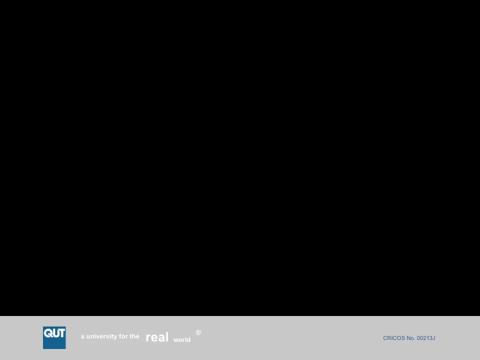 we can do element wise comparison operations: Greater than, greater than or equal to, and so on. If an element is compared with another element, the result is false, Then it's assigned a numerical value of zero. If it's true, it's assigned a numerical. 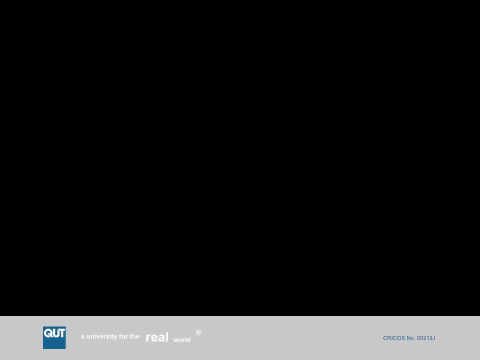 value of one. If we do arithmetic between a matrix and a scalar and what MATLAB will do is for every element in the matrix it will perform arithmetic with the scalar. So if we do a matrix plus a scalar, it will add the scalar to every element in the matrix. 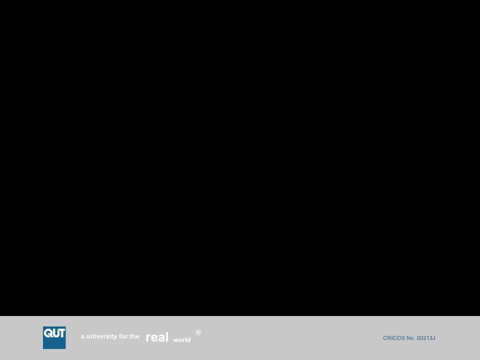 If we multiply a matrix by a scalar, every element in the matrix will be multiplied by that scalar. If we compare a matrix to a scalar, we compare every element in the matrix with that scalar and put the result into the corresponding element in the matrix on the right hand side of the